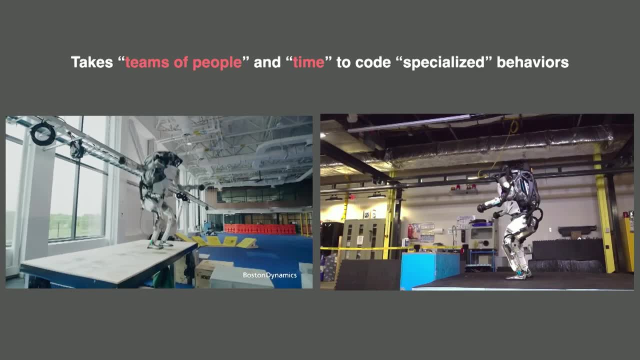 It might be months to a year, maybe more, to get to one behavior. So if you're interested in coding up many behaviors or many tasks, the scheme currently is just not scalable. So that leads us to the goal of being able to quickly and 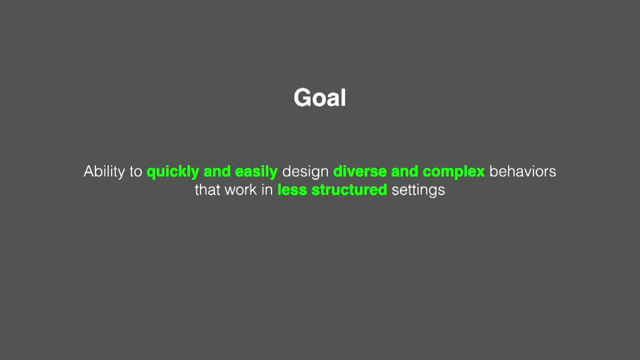 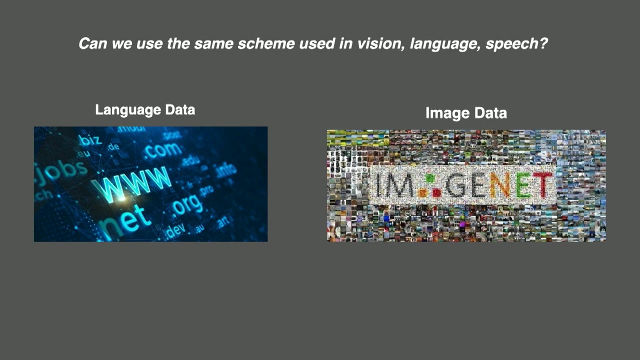 easily design diverse and complex behaviors that work well in less structured settings. And the one question you can ask is: well, can we use the same scheme that we had in vision, language and speech? In these domains, we had tons of data. 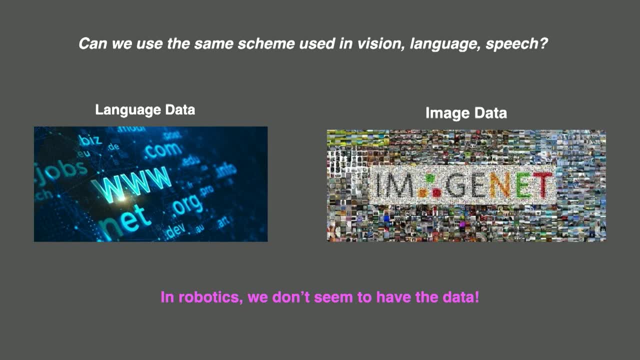 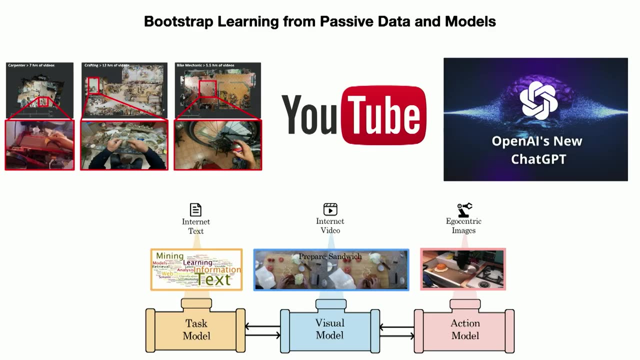 But the problem is in robotics we don't have the data already lying on the Internet that we can download and train these large models. So what are people doing? So there's one line of work which is trying to bootstrap learning from passive data. 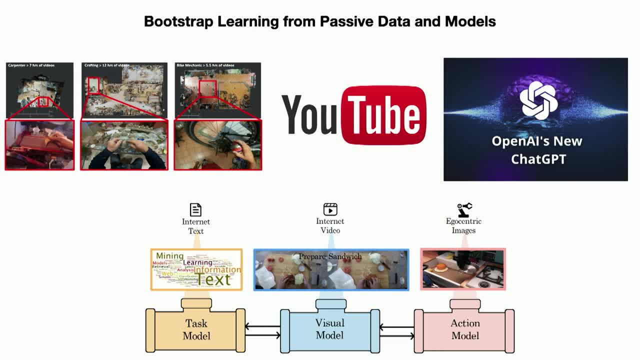 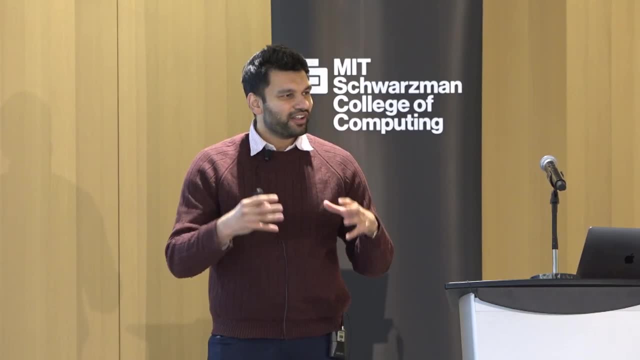 For example, data available in terms of YouTube, by leveraging models that people have already trained, For example, language models, vision models, putting them all together- And this is an exciting area, But for today, I'll focus on really collecting robotic data. 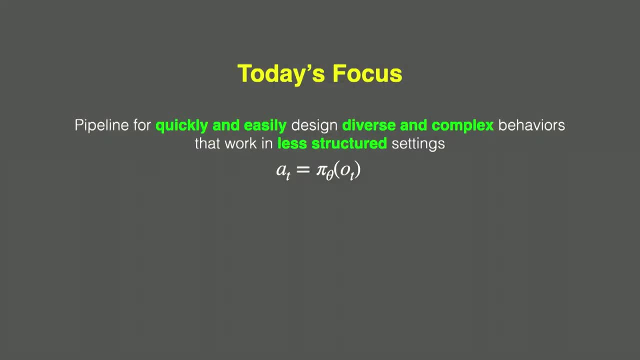 And what do I mean by robotic data is we pick up a task and we say: do I have a controller which is going to take in observations and map to actions And if we can design a framework which allows me to do this for many? 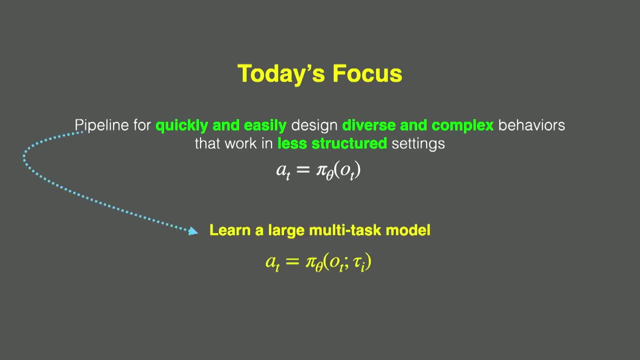 many tasks and very quickly. then essentially I can train a multitask model Where over here TI indicates a particular task, And once I have this multitask model which I can start training, this in turn would help me design controllers for new tasks faster. 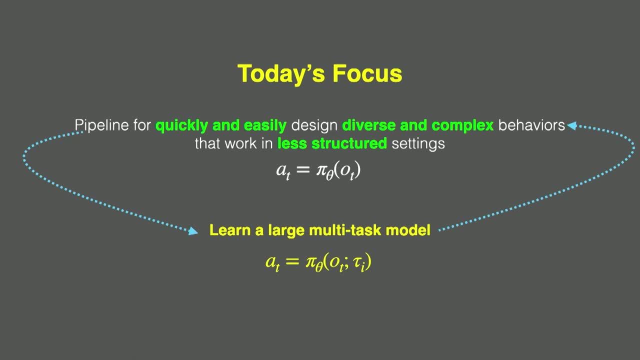 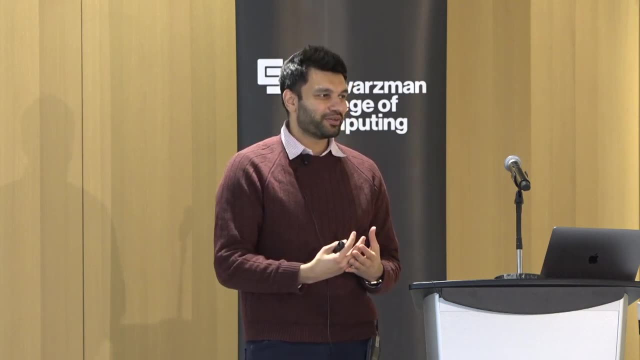 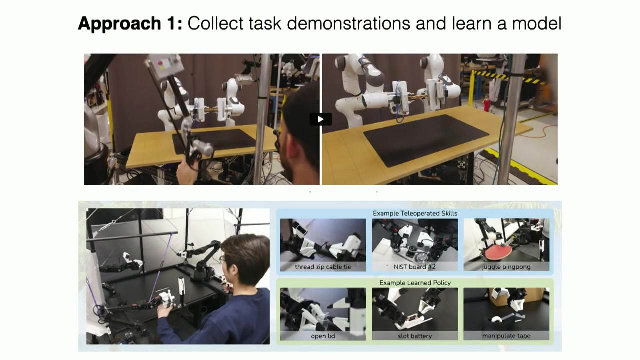 So the core question really is: how can I take a new task and design a controller Very, very fast? By very fast I mean human time, wall clock time, the amount of effort which goes into it. So I think in the field there are pretty much two approaches. 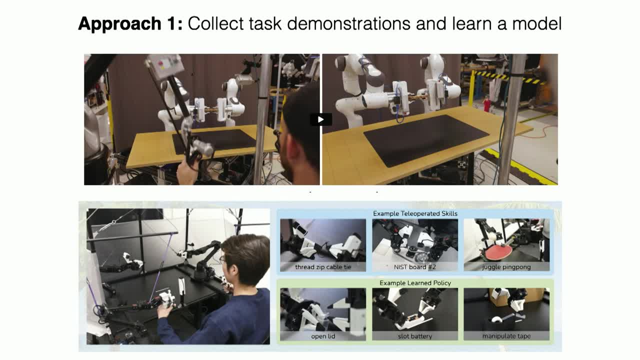 which have emerged to tackle this sensory motor problem. So one of them is collecting large demonstrations, And there are many groups at ERI, at Stanford and at Google which have done teleoperation and showed some impressive tasks that they're able to perform. 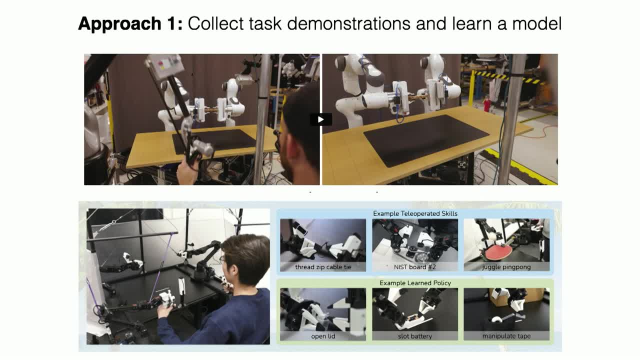 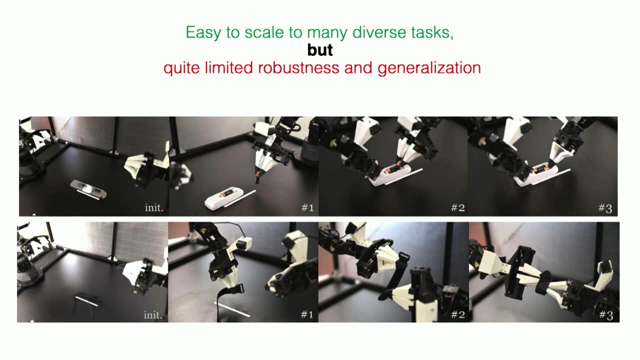 So the good news about tele-operating the robot is that you can pretty much have a robot do many different things. But if you look closely at the kind of demonstrations that have been shown, for example over here, putting a battery in this socket- 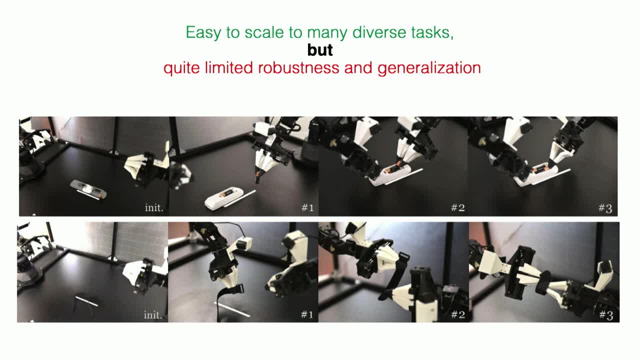 You see this white line which has been drawn over here, And this will only work if the object is placed, and so placed around this white line, The point being, these systems can do complex tasks, but they're not as robust as we would want them to be. 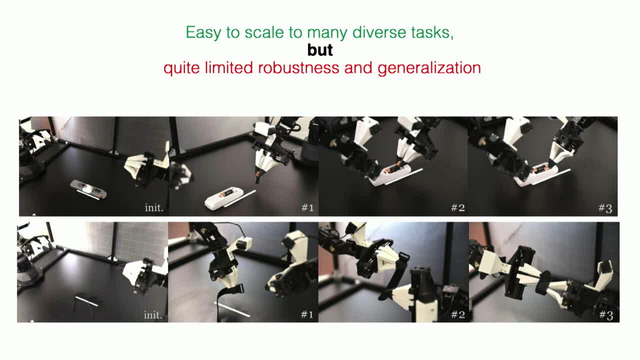 They're not generalizing. And you could make them generalize, and what that would mean is you have to go and collect more data. So the data effort over here comes down to how much human time and human effort is required in collecting the data. 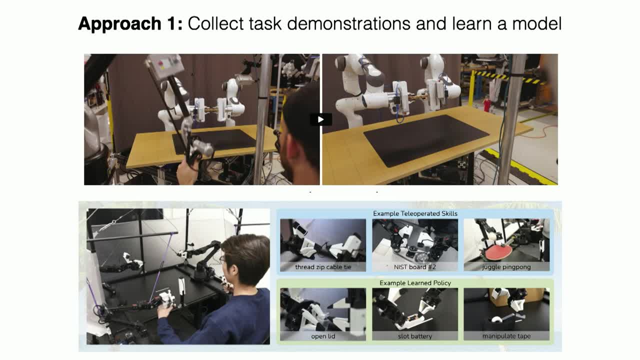 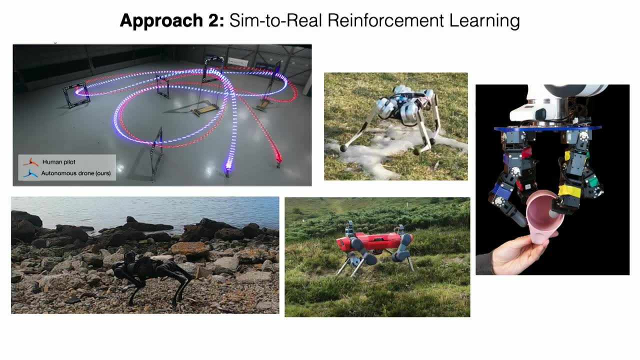 And this is what people end up doing: They have these two arms and they're trying to control the other two arms to collect more data. So the other approach which has become quite popular is sim to real reinforcement learning, And there have been good results on a broad variety. 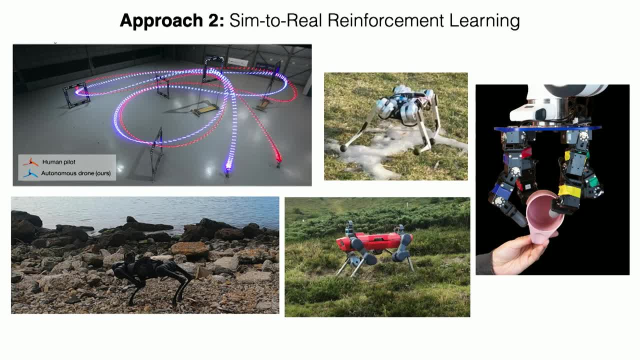 of platforms. This is a photo from a Nature paper showing how automatic drones, or drones learned with reinforcement learning, can beat the fastest human player. There are a bunch of works on quadruped locomotion and also on dexterous manipulation, And while this sim to real reinforcement learning, 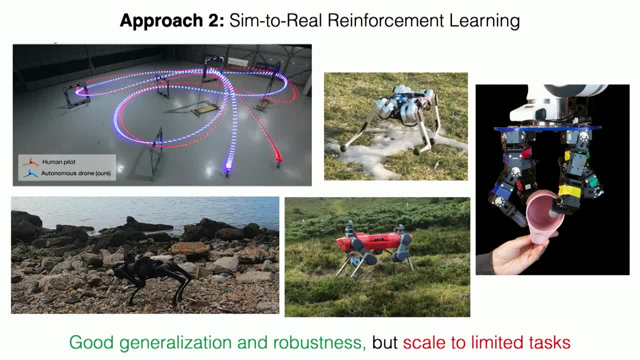 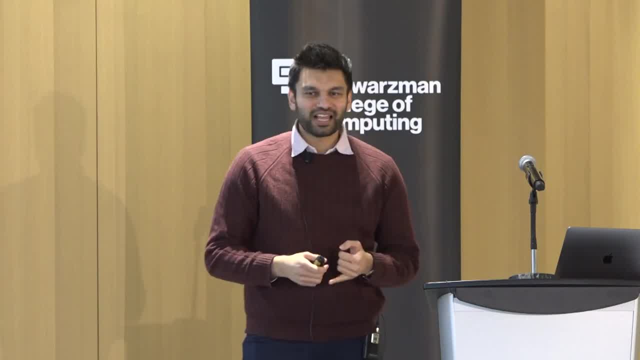 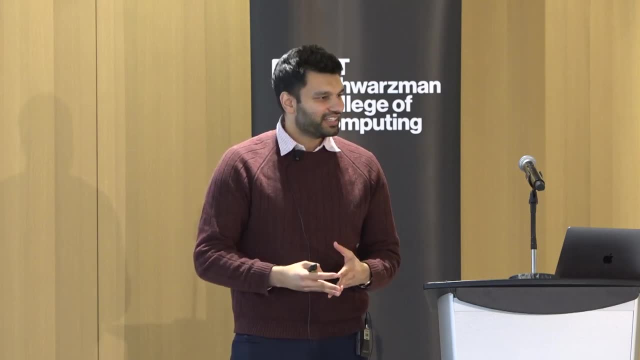 can get good generalization and is more robust than what you get by collecting data manually. we cannot scale this to many, many tasks, because there are a couple of challenges. For example, you can only go to tasks that one can simulate, and there are other issues which come in. 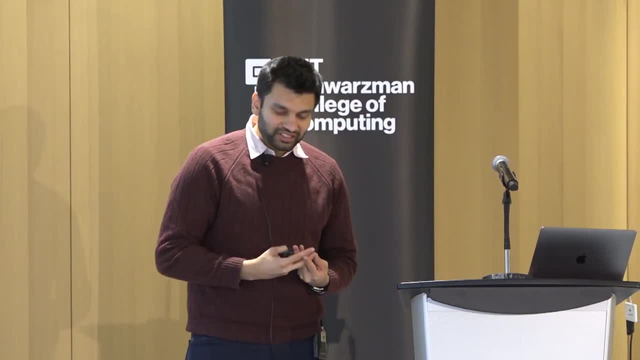 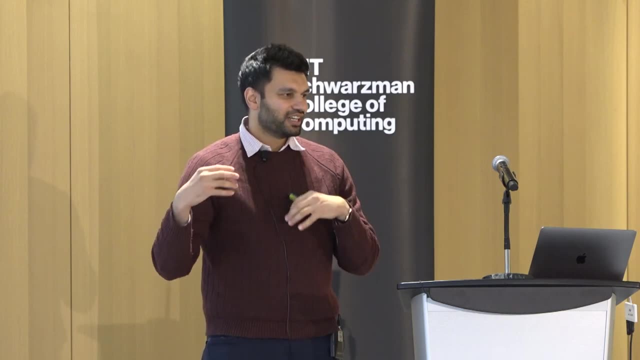 So, in a nutshell, I think the question really we should be asking is if we have the approach of either teleoperating the robot or this approach of going to a simulator collecting data in the simulator. what is the quantum which really matters? 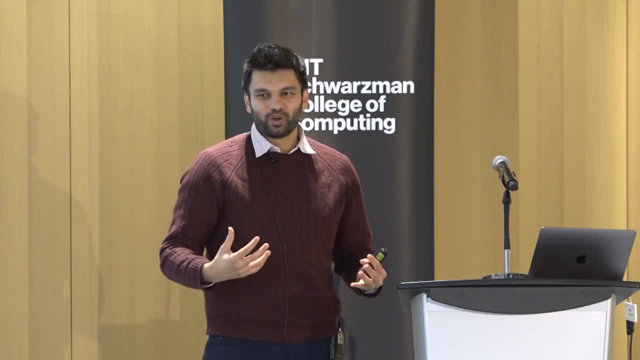 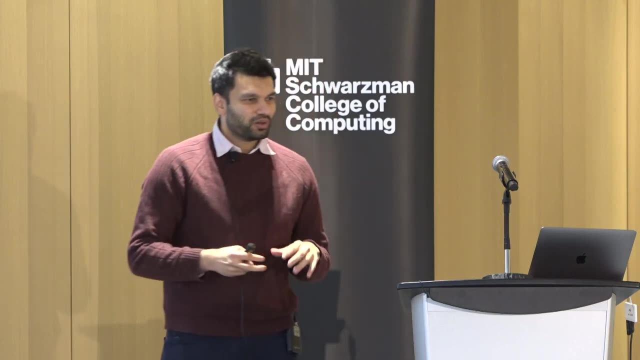 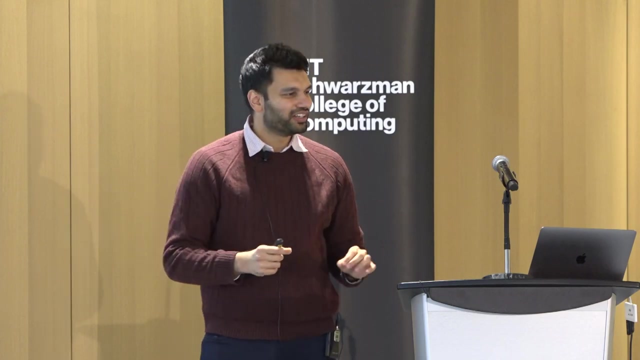 And in some ways that is the amount of human effort and time which goes into setting up these systems so that we can come to a controller. So, in line with the theme of the session, I'll fixate on the sim to real reinforcement learning. 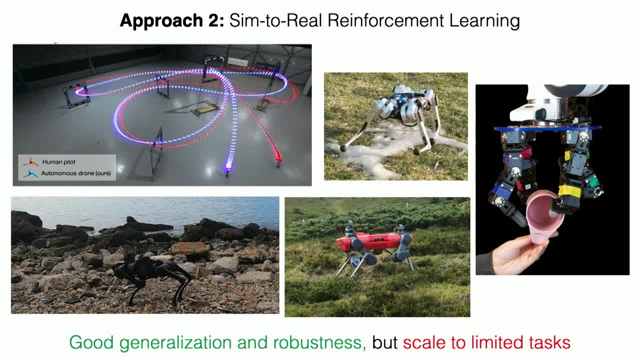 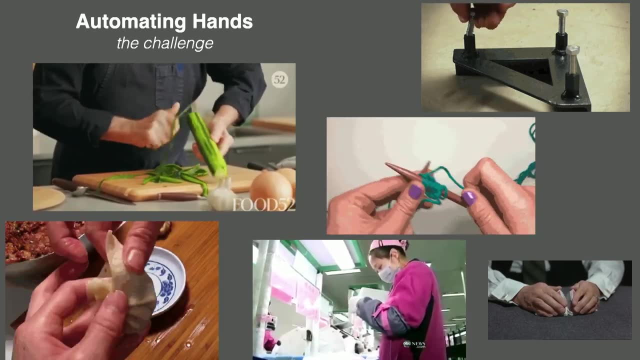 and tell you where we are highlighting some of the work that we have done and what are some of the issues which are preventing us from scaling as fast as we would like to scale up. So, for example, one thing we would want to do. 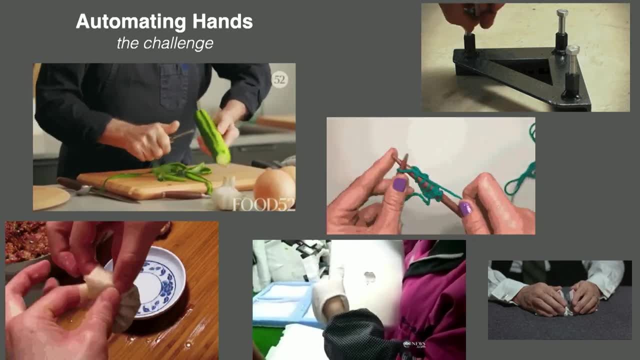 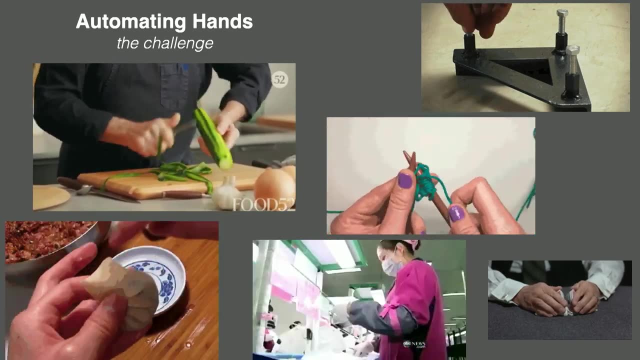 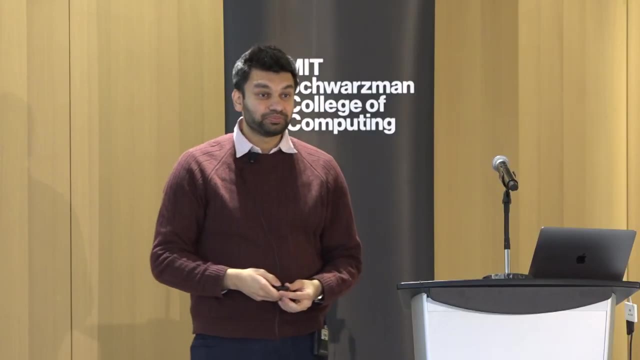 is to automate many of the tasks that the human hand can do today, And the core part of many of these tasks is that there is motion between the hand and the object, And that is what distinguishes this from purely picking up an object and placing it. 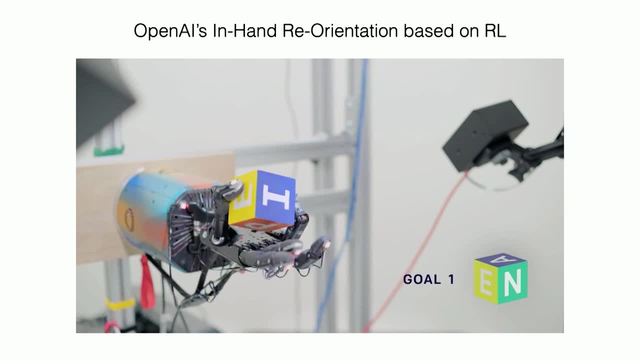 So OpenAI had this nice work back in 2017 where they were demonstrating a hand can rotate this cube And they had a camera looking at the hand. But if you actually look at this system, the setup, this is what it looked like. 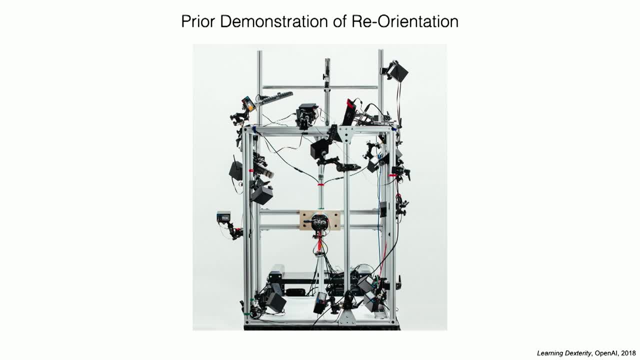 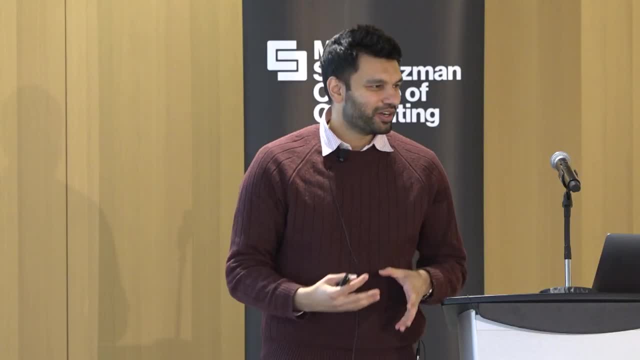 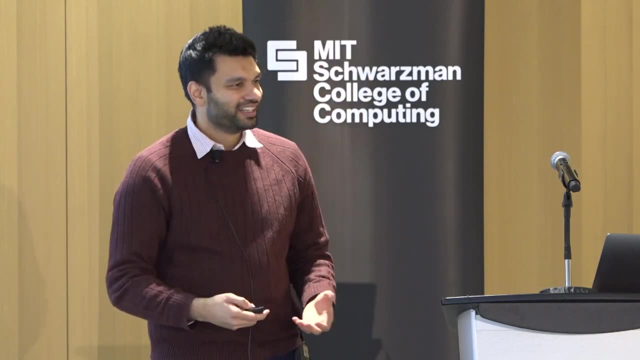 It had so many cameras to make this happen, so that the state of the object and the hand can be measured accurately. So very good for a lab demo, but not really practical, And furthermore the system only worked for one particular object, which was the cube. 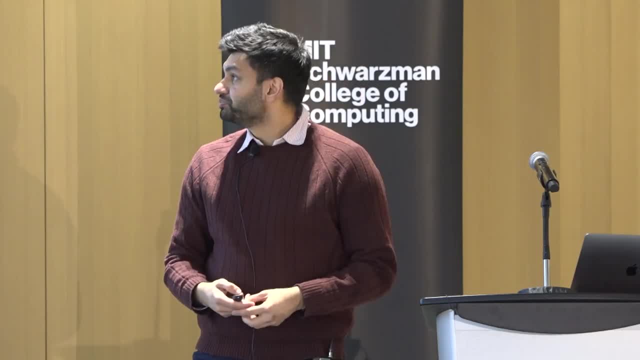 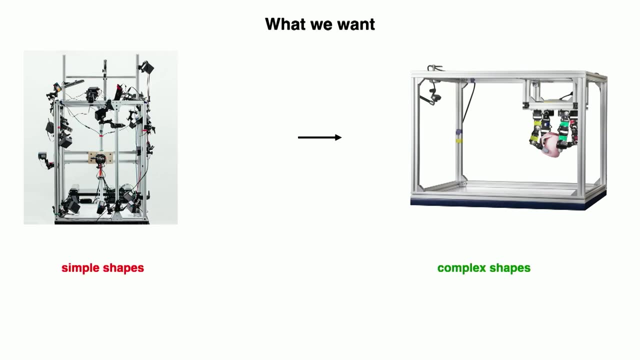 So it's not generalizing and seems impractical. So the one thing we set out to do is: how can we get to a reorientation system which can work for diverse and complex shapes and also generalizes to new ones, while having a setup which is much more practically deployable? 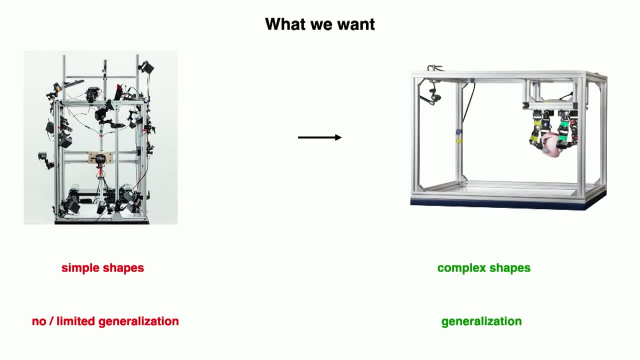 For example, having a single camera. look at this four-finger manipulator: manipulate an object, And this was work led by Tao Chen in the lab, And the way it works is we go in a simulator and we collect large amounts of data. 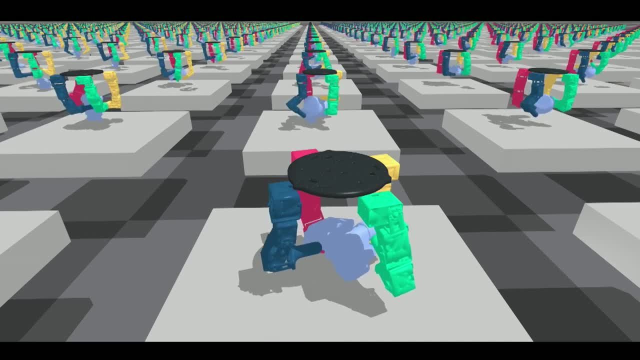 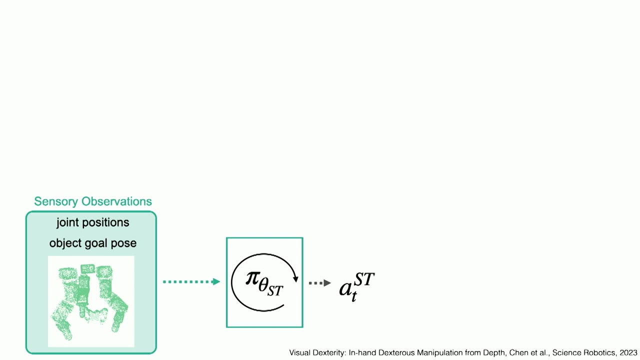 And this is possible because we can run many, many environments in parallel, And what you see is the hand trying to manipulate many different objects. So, ideally, what we want, the end result, is a policy which can take in a vision, observation or a point. 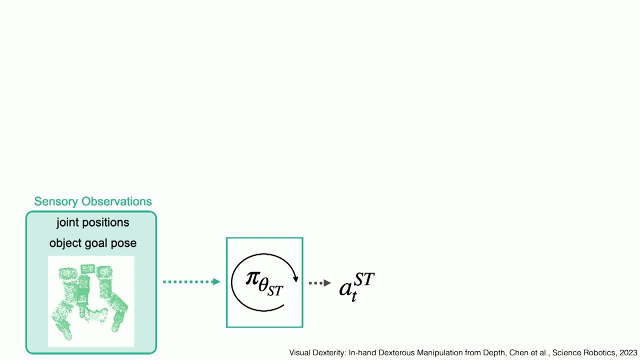 cloud coming from a camera where the fingers are, and then output actions so that we can complete this reorientation task. Now it turns out that if you try to train reinforcement learning policy from a high dimensional observation space, it's actually quite hard to do it. 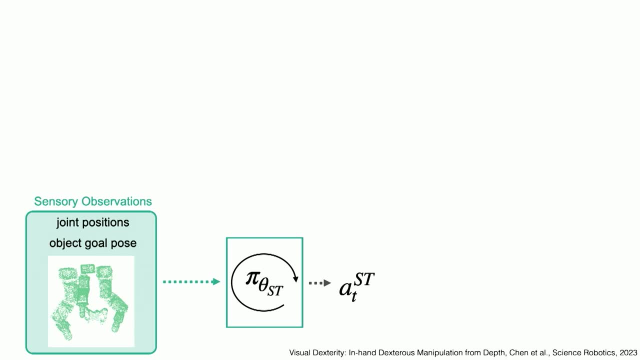 And the second thing is doing rendering in simulation can become quite challenging, So these kinds of policies just do not work out. The framework is: there's a camera getting observations, There's some rewards that we define, which is RT, And the rewards might be how close we are to the target. 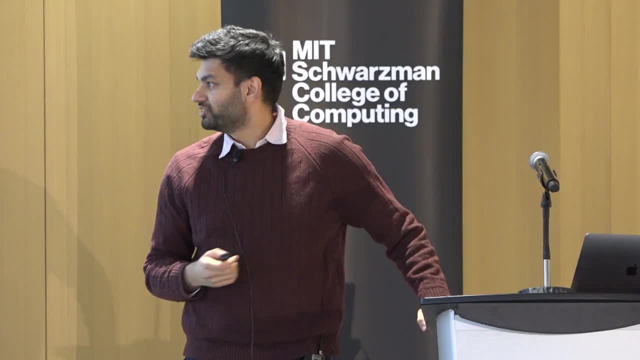 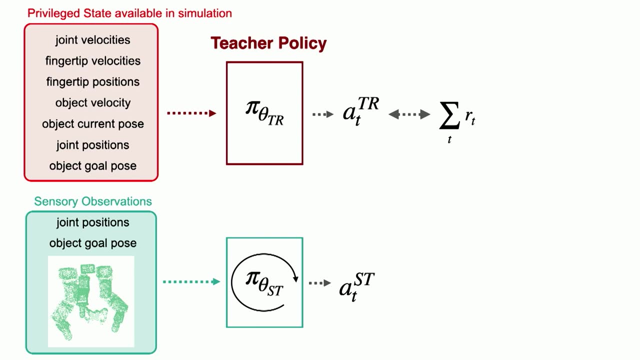 And we want to maximize the sum of rewards. It turns out it's very hard to train these policies, But in simulation you can play God and leverage the fact that we know all the information about our environment and the object. For example, we know the object pose. 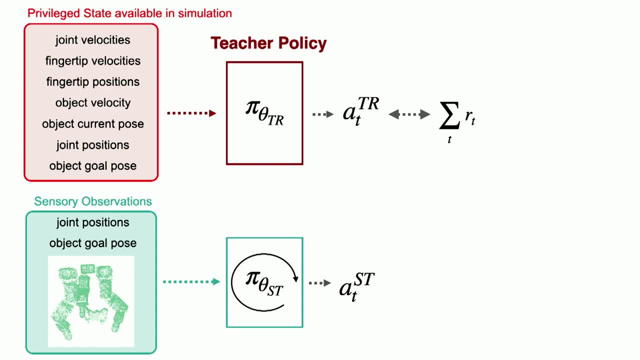 We know the object velocity, And this helps us construct a reduced state space. What I mean is this is much more lower dimensional than the observation space on the bottom. Now, if you study machine learning, one of the basic things is that if your observation space is, 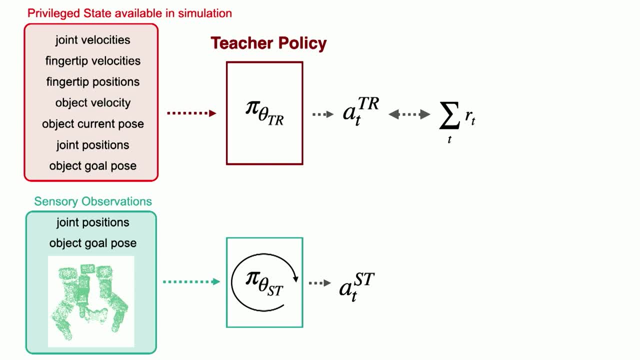 small, it's much more easier to learn a mapping than if your observation space is much larger. So by leveraging this, we first train a policy using reinforcement learning, which we can do now easily, And then what we do is we distill this policy. 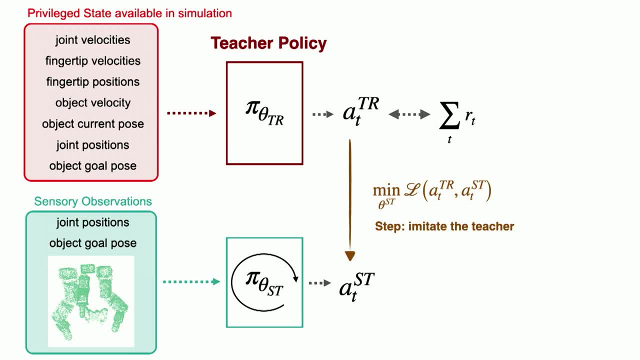 to work from sensory observations. So step one, use reinforcement learning. Yes, learning, train the policy to do reorientation. But this policy we cannot deploy because it already assumes object velocity, pose and this kind of information which needs to be inferred from sensory data. So to make that possible, we take sensory data but we get 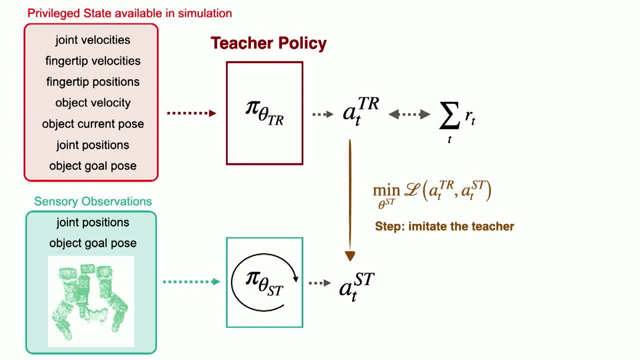 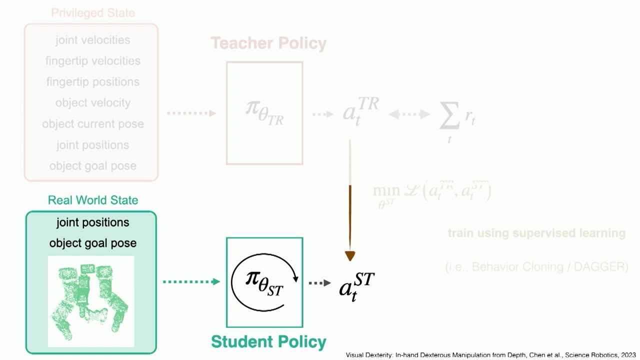 targets coming from the first policy And just to supervise learning, to learn the policy on the bottom, And this framework is called the teacher-student framework, And then we can take the second policy and deploy it on our best scenarios. So here's an example. 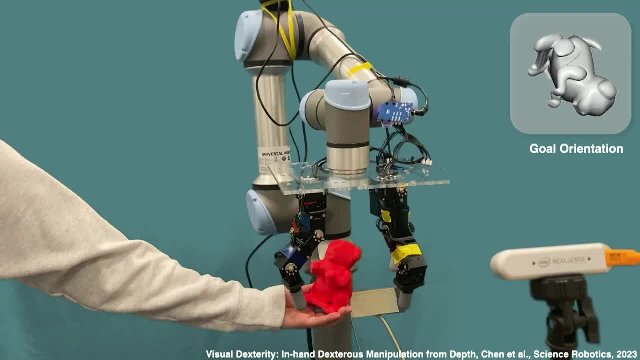 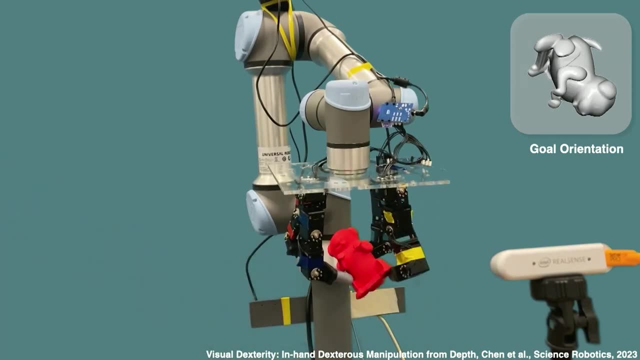 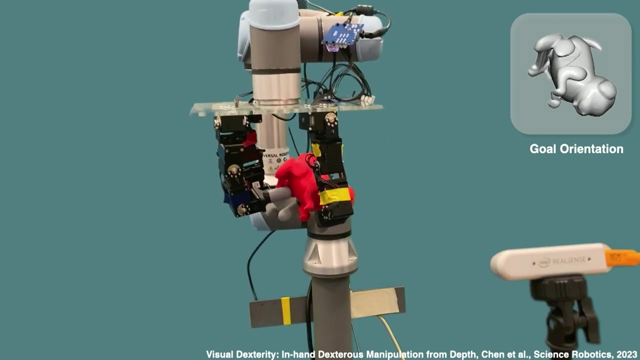 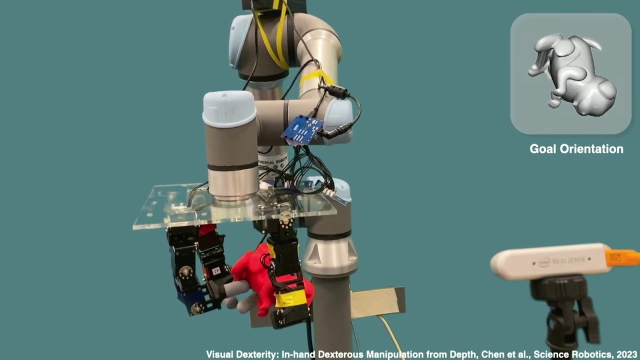 where there's a camera looking at the object And this is the orientation that we want to get the object in. So let's see what the system ends up doing, And what you find is the system in orientation. So it takes this object and takes it to the target orientation. Now these are objects. 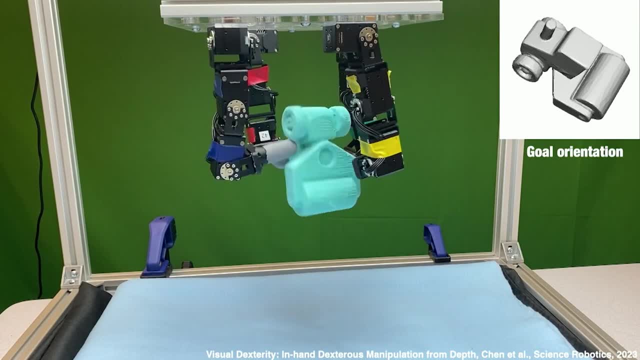 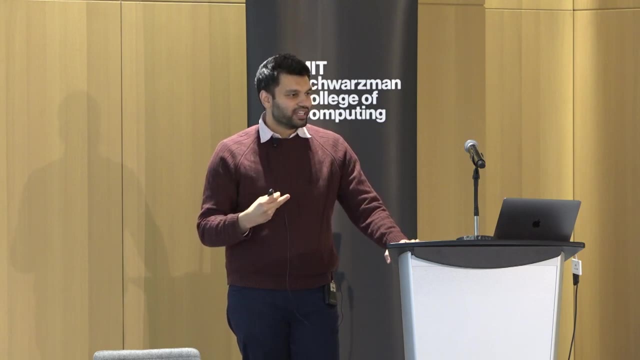 that the system has not seen before. Here's another example of trying to orient the object to the goal orientation. So the system is not perfect. It is still imprecise in terms of how precisely it can rotate the object, But at least we are showing evidence that. 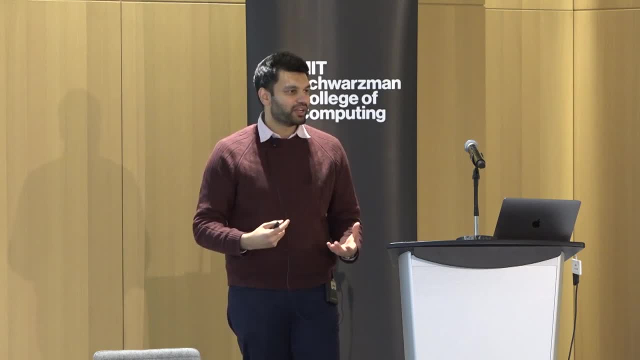 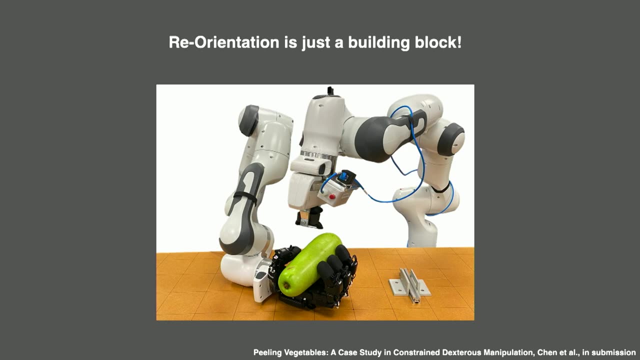 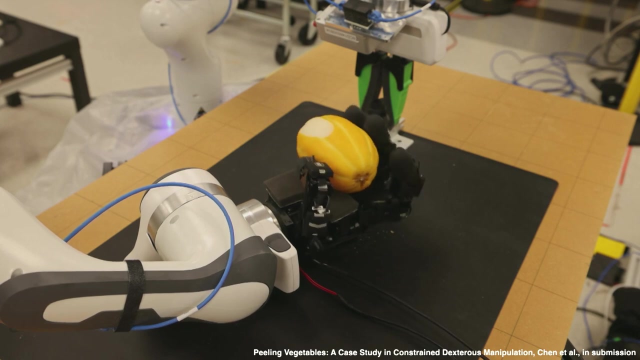 we can go to complex objects and perform this in-hand manipulation task. Now, once we can start doing it, you know we can start leveraging these controllers for more tasks, right? For example, peeling a vegetable over here, where the vegetable needs to be rotated. So now I can have this vegetable that I can reorient. stop when I see. 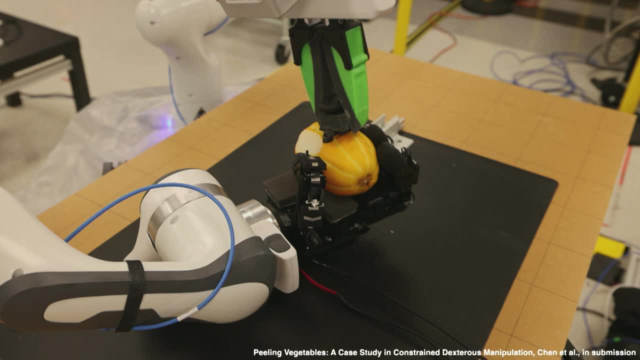 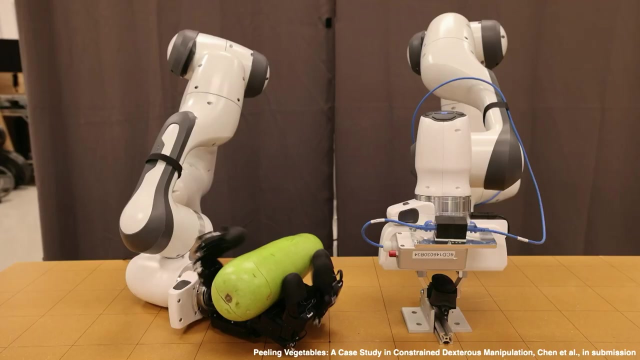 the unpeeled part, And then there's a second hand which comes and peels it. At the time we clicked this video, this was being tele-operated, But now we have automatic systems which can also, you know, do the peeling. So I think this opens up like a nice space for actually. 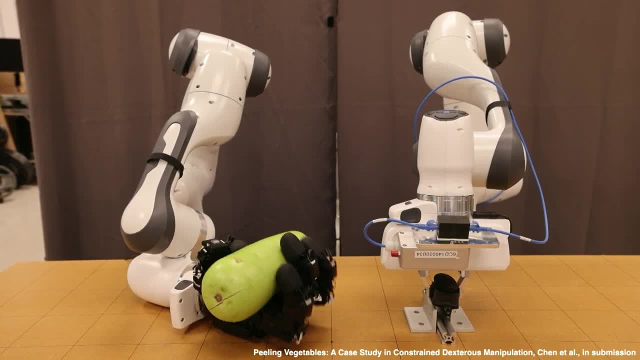 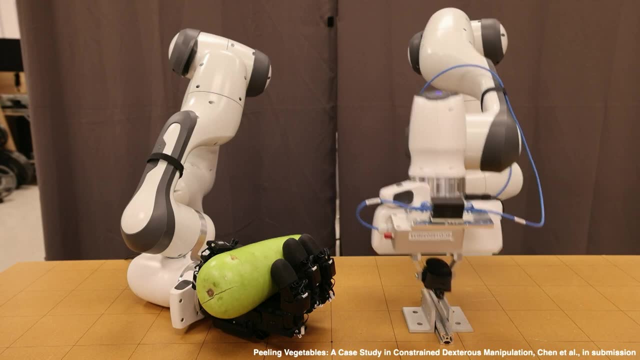 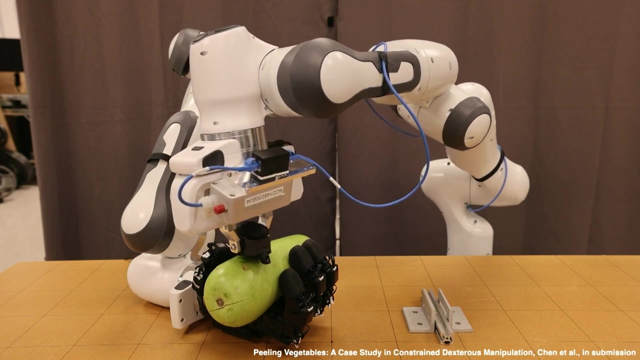 picking up tools and trying to use them for bi-manual tasks, and which could enable interesting advances in manufacturing, but also for robots to become more versatile. Here is just another example of applying it on a different vegetable, to make the point that we're not limited to just one or two vegetables, but we can bring in new ones. 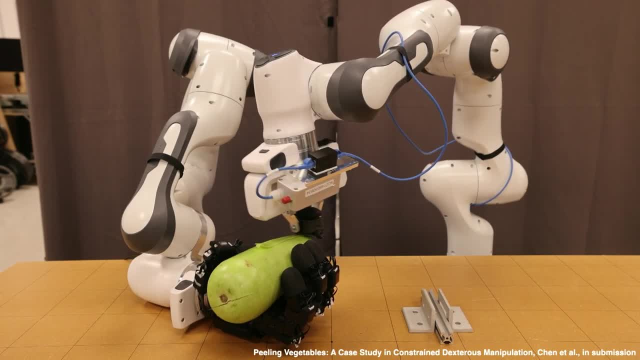 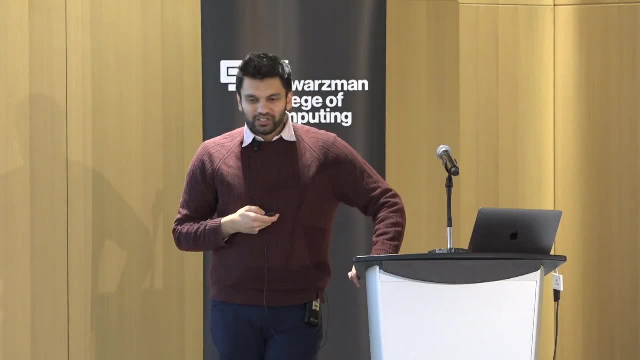 You know, not ginger yet. you know, but that's where we are going. You know, can you give a ginger and then have a robot actually peel it? Now the good news: with the framework I just described to you, which is collecting data, 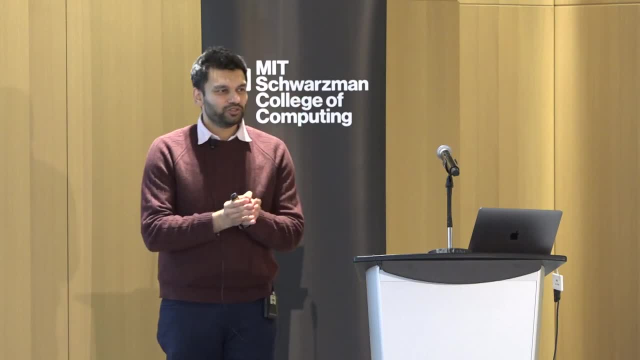 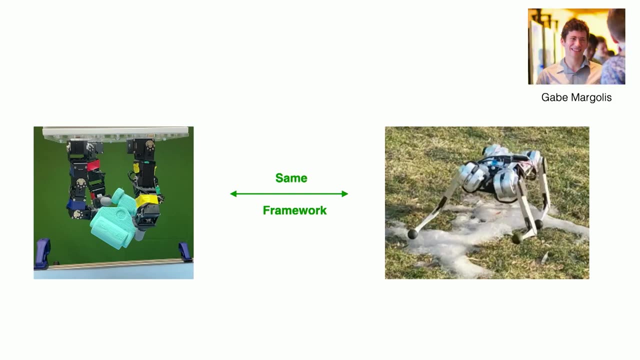 in simulation and transferring to reality is that we can use the same code base, pretty much the same framework, and apply it to different tasks, You know. so I'll show you some results now, in locomotion, being pioneered by Gabe Margolis, who is a PhD student in my lab. 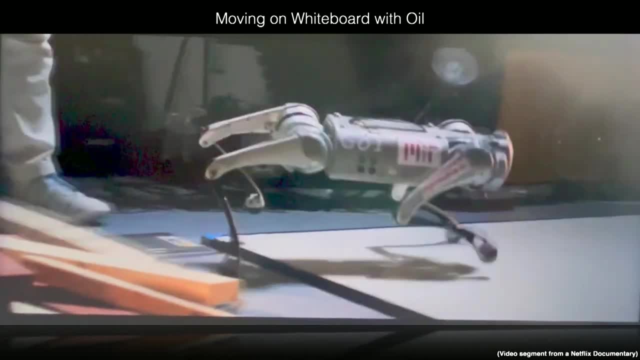 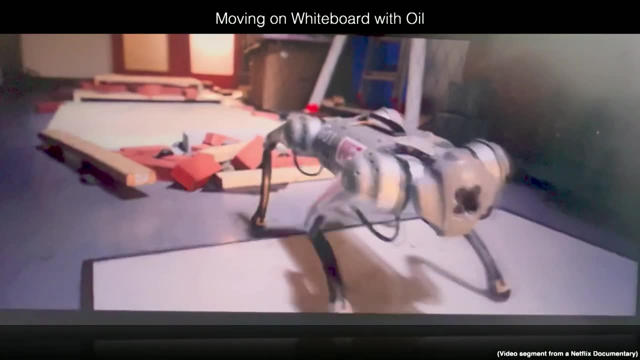 So you know, what we've shown is that the policies that we end up learning through sim2real learning end up being quite robust, because we can emulate many different scenarios in simulation. You know, here's a robot. you know slipping over oil, but it you know. 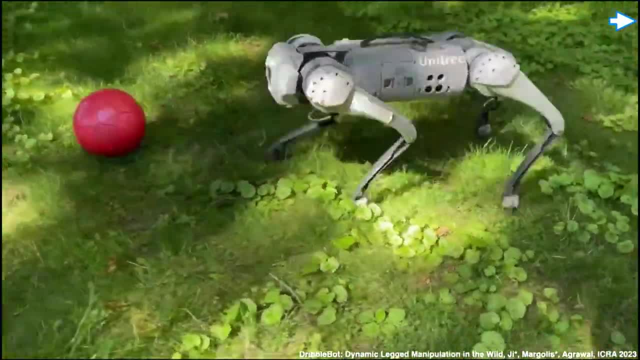 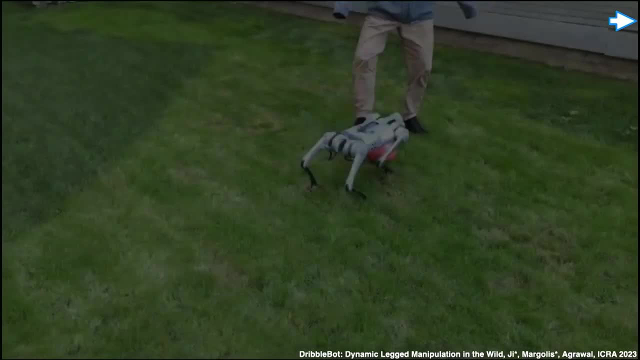 remains robust. You know, once the robot can walk, we can make the task be more challenging. For example, now it needs to kick the soccer ball, so it needs to balance on three legs, while using one of its legs to dribble. 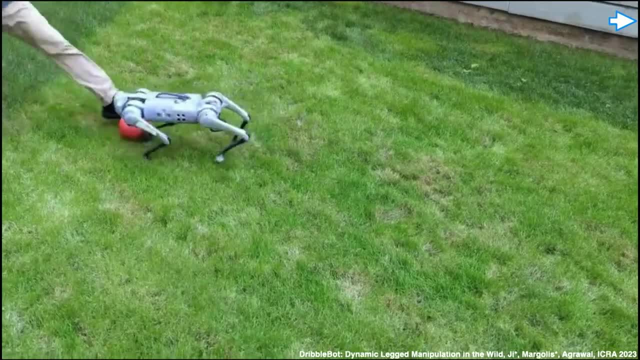 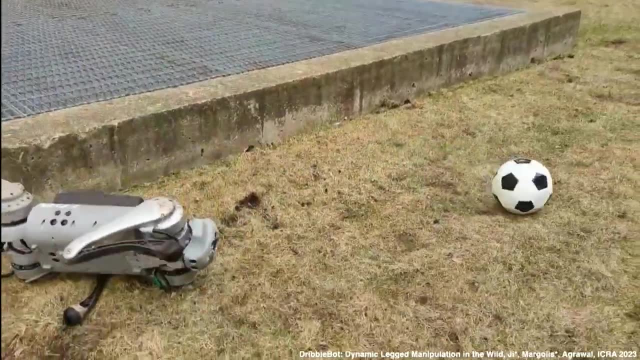 And the human over here is pretty much a nuisance. you know trying to, you know, get the ball away from the robot. You know these policies, you know, again by the virtue of collecting lots of data, are robust so that the robot falls down. it will get up and continue. 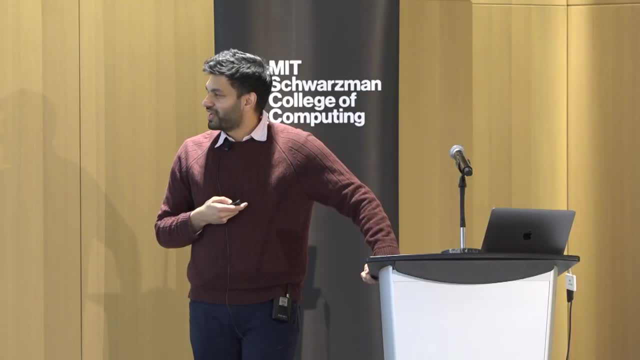 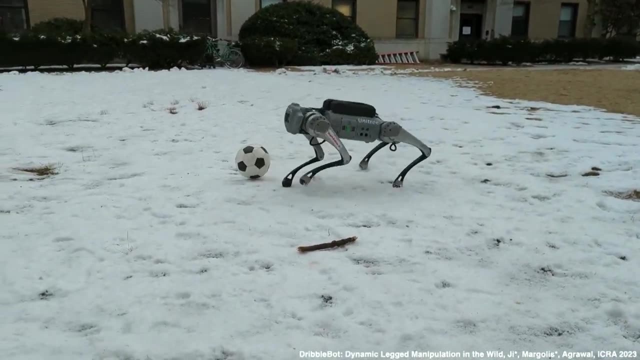 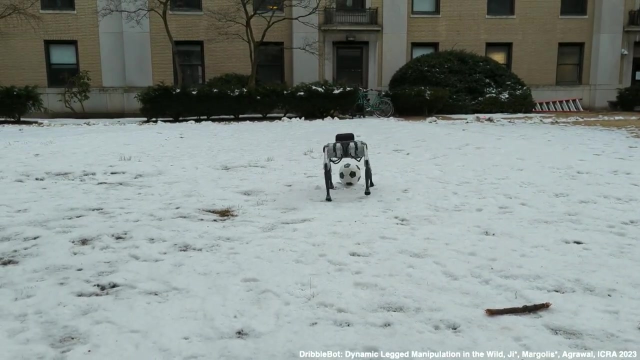 dribbling the ball. You know, one thing I didn't realize before I moved to Boston is how much fun snow can be for robots. So we can take robots out and really test, you know, their robustness. There are a lot of scenarios which can become quite challenging, right? So here is you. 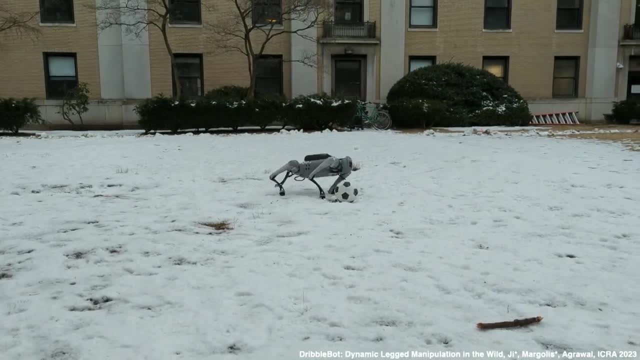 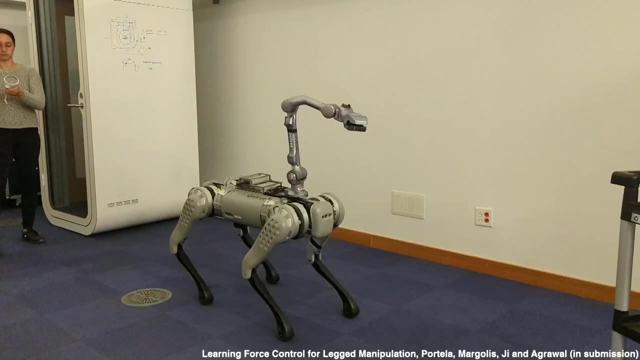 know a robot trying to dribble in snow. It's struggling But, you know, at least it's trying to get its job done. Now, once we can dribble, you know, we can also, you know, put an arm on the robot and 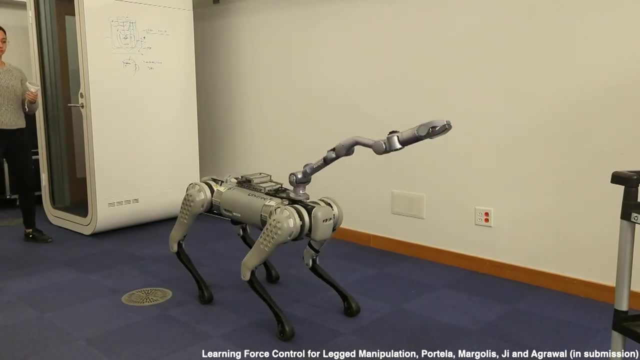 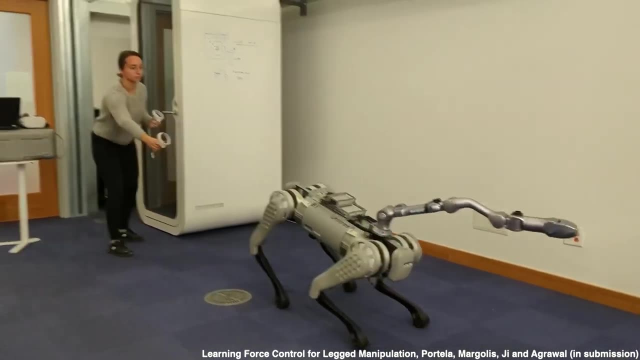 have the arm go around. So here we are teleoperating the system, or Tiffany is telling the way the end effector should go And the robot uses its body To follow and make the end effector pose be possible. Now we can not just do positions. 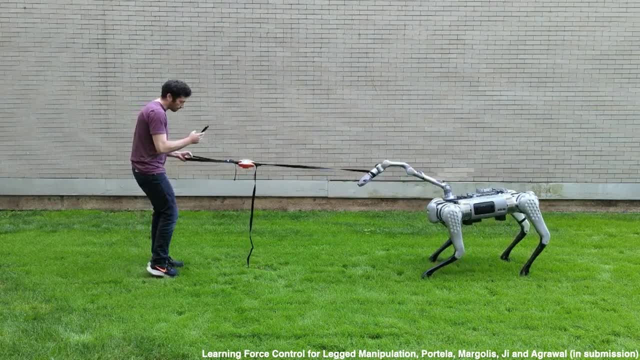 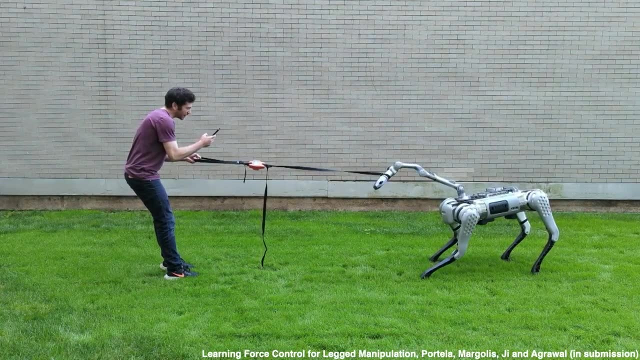 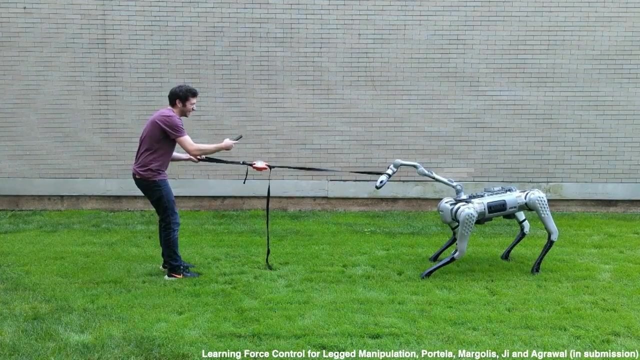 but we can also do this with forces where, over here, Gabe will try to pull the robot and what you'll see is the robot will adjust its hips to try to increase the amount of force it can apply, right, And now Gabe is really struggling. Now, once you can do you, know force control, Oops, I had some videos, but I think it was very successful. We can go one step closer to get the robot going, But the goal is to keep the robot in a position. So now you have a robot that can go up, it can go down and it can go up with a motion. 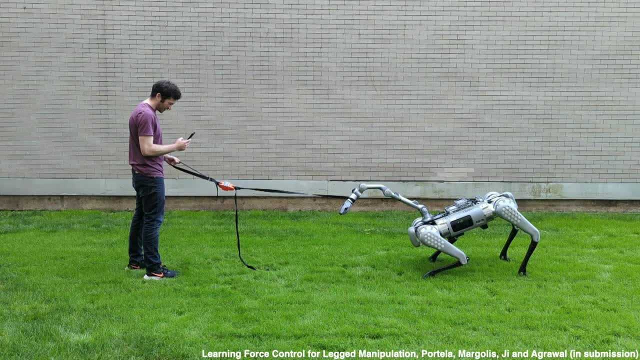 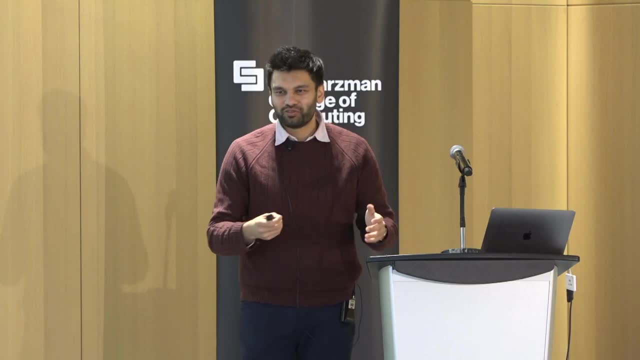 some videos, but I think I skipped one of them. it means that giving you know demos become very easy because you can just with one finger- now you can move the gripper of the robot and it will follow what you're doing. So you know what I. 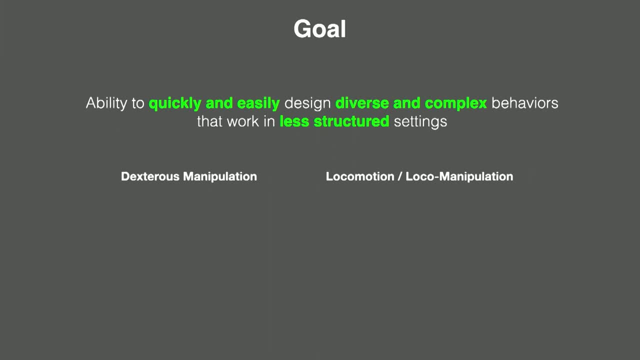 have shown you is. you know some examples in dexterous manipulation and locomotion, where we are able to design behaviors using the same framework. So these tasks are complex and we are showing that they're working in less structured settings, but there's still challenges. and how quick and easy is it to design? 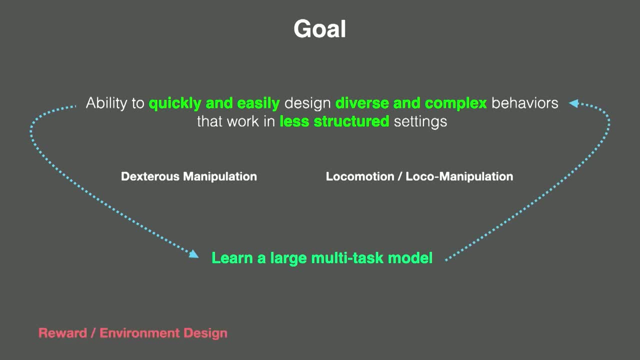 these behaviors right. So some of the challenges really are that one needs to spend substantial effort in designing the reward function and the environment, you know. the second challenge is: what can we actually simulate? and the third challenge is: you know, how safe are these controllers when we actually deploy them? 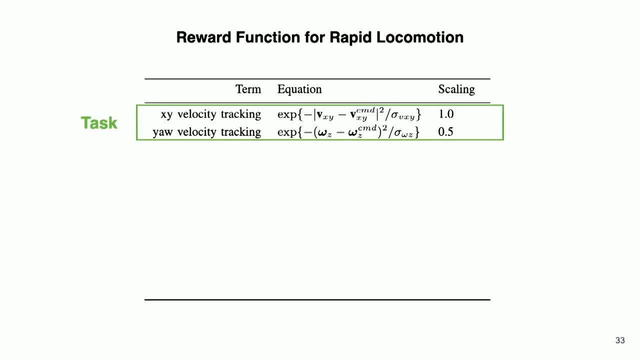 So first, you know, I'll chat about this problem of reward design. So when I was telling you about this robot which is a robot, which is a robot, which is a robot which can run in different scenarios, you know what you would expect is- I gave a. 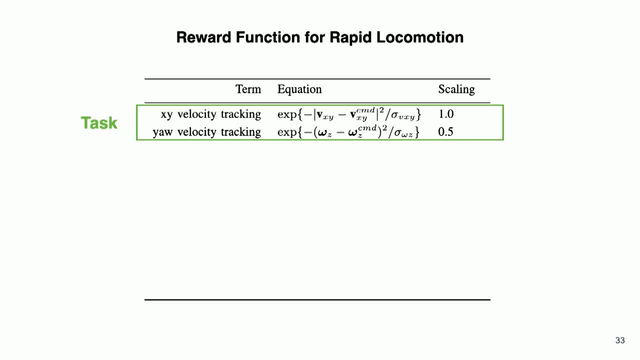 reward function, which expressed in the velocity that we want in XY and maybe how much velocity I want the robot to turn. But this turns out to be insufficient and people typically add more terms to it, right, For example, things like: you know what should be velocity in the z-axis? the base should: 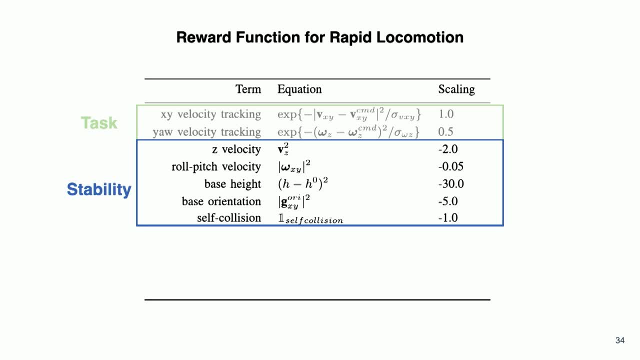 not be too low. So you're trying to help the robot discover particular parameters, right? And then there are some terms they should not be here, but there's some terms which are trying to, you know, make the robot's behavior be smooth by penalizing energy. Now, coming up with these terms and coming up with these, 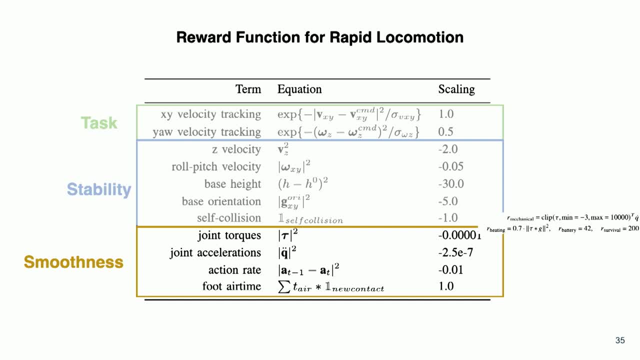 coefficients is what you know. people spend up, you know, quite some time designing it right. So we would ideally want to get rid of this right. So how can we, you know, reduce this effort? So you know what I'm going to tell you is you? 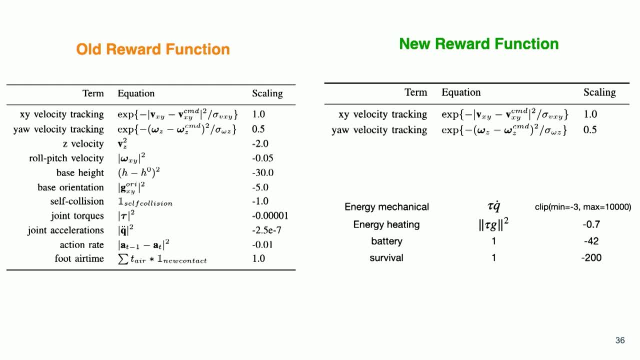 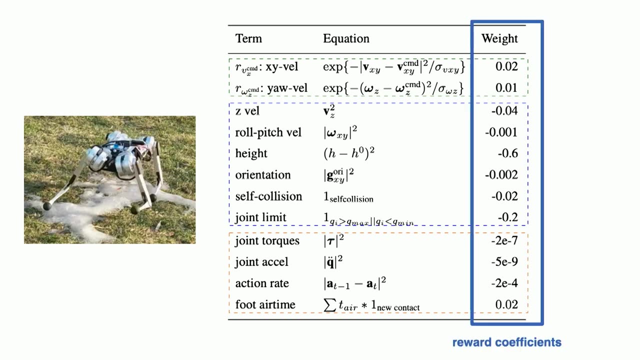 know, we have an approach by which we can go from this old reward function to a reward function which looks, you know, much simpler and but still retain, you know, many of the same properties, right? So how do we go about it, right? So let's first consider the question of that. someone came up with these terms, but we 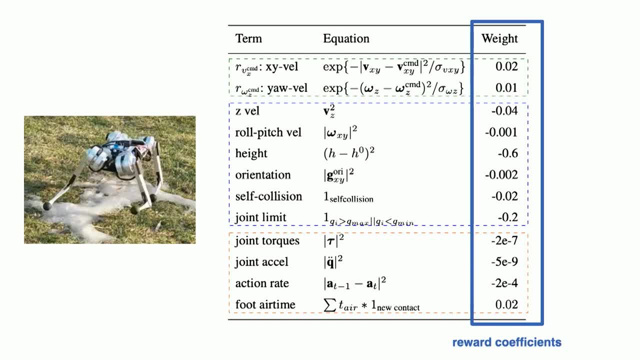 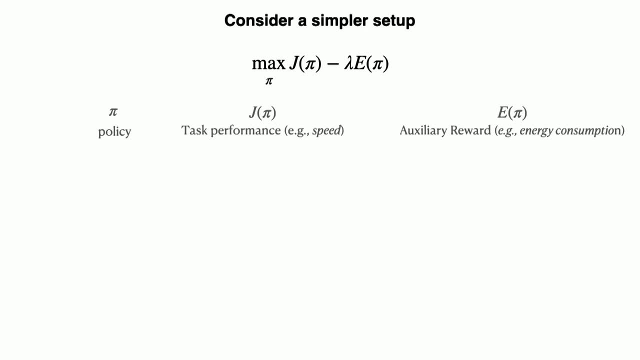 still want to find these reward coefficients automatically, instead of someone setting them by hand. Maybe I have two minutes, Okay, So now consider this problem set up where I want to maximize my task performance and I want to minimize the amount of energy consumption, which is 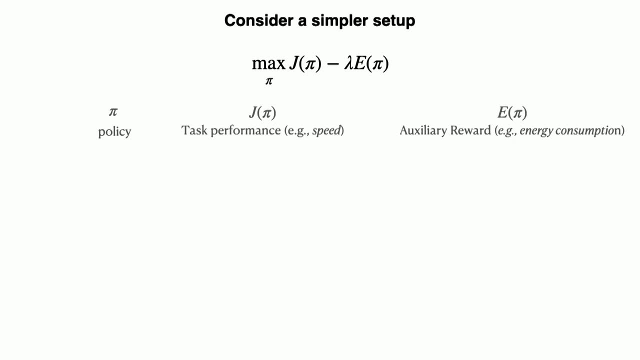 happening. And then I want to trade them off with this parameter lambda which says: you know how much I prefer one term versus the other term. Now I can plot energy versus the task performance, and what I want is to be very performant at the minimal energy expenditure. So now, if we end up, 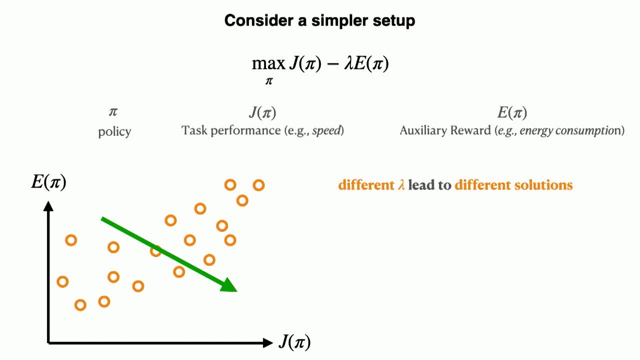 choosing different lambdas. this ends up corresponding to different dots over here. So ideally, what I'll want to find is what people call the Pareto optimal, which means that if I am getting a particular performance and a particular energy, I cannot improve my performance without increasing my energy expenditure. 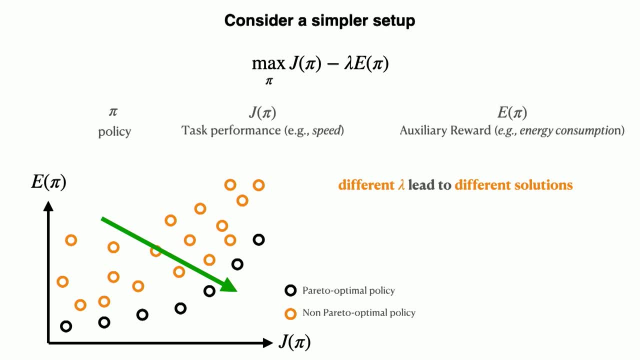 Those are the kind of points that we would like to find. So you could do it by doing a hyper parameter search on lambda, but that ends up being quite expensive and this is what people end up doing by hand. So we try tackling this issue, and the way we do it is to say: well, you know, let's learn two policies. 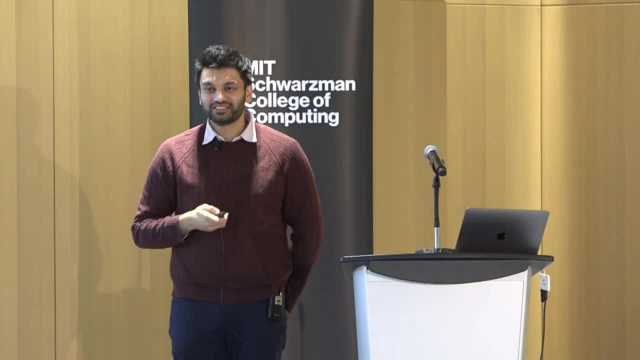 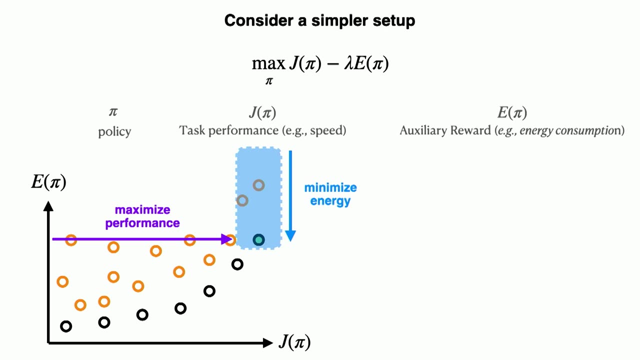 and let there be a game between these two policies. So one policy goes and tries to maximize performance and the other policy is going to minimize energy And hopefully, when these policies are fighting, we're going to find, you know, something close to the Pareto optimal. 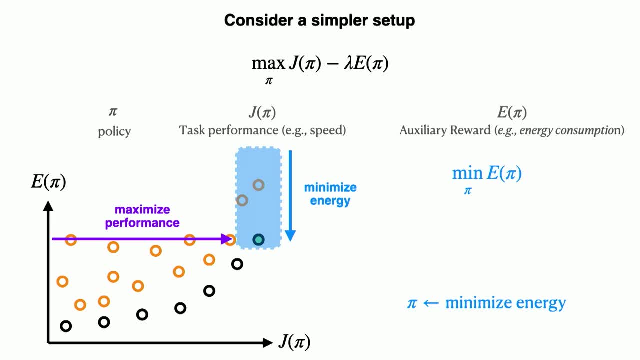 So we have one policy which is trying to minimize energy and the second policy which is just trying to maximize speed, And then we couple them with a constraint and the constraint pretty much says that, you know, the policy which is minimizing energy should get as much reward as the policy which is only 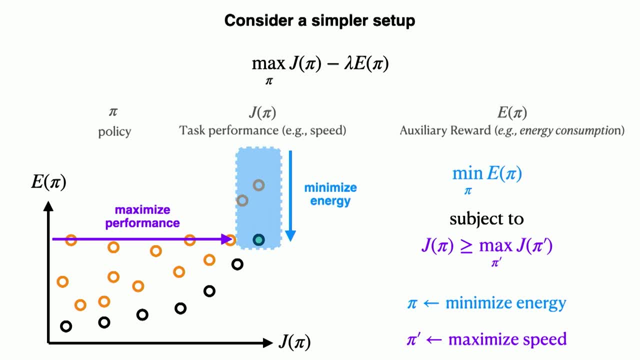 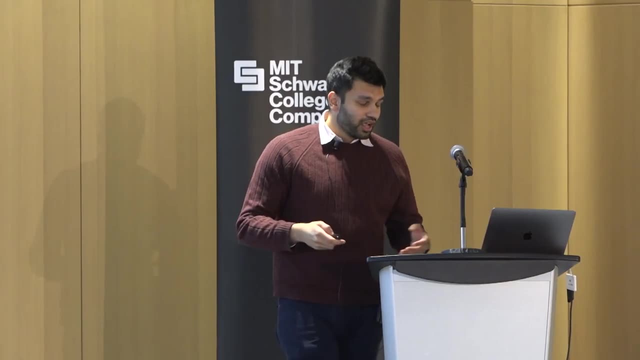 trying to maximize speed. So what you're saying is you're trying to push- you know the policy- to get more reward the speed one, but you're never letting the energy one be less performing. So trying to push energy while still trying to maintain performance. Now, if we end up doing this, you know we can. 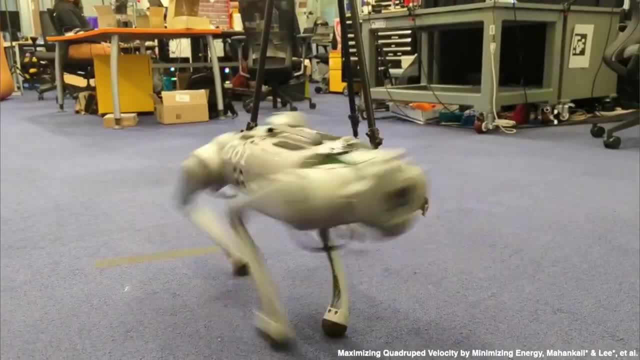 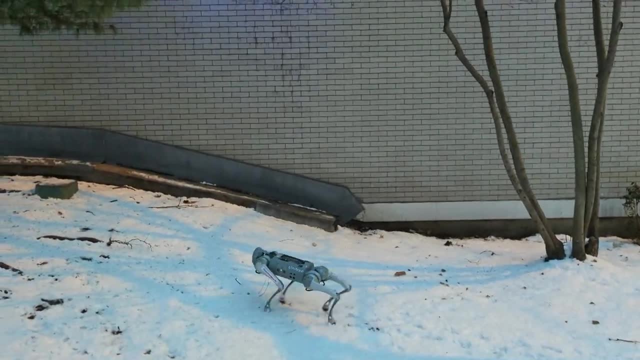 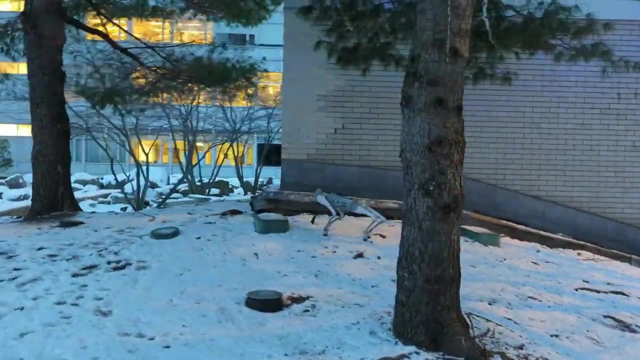 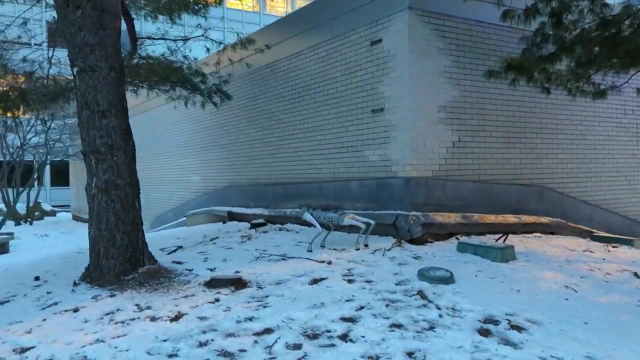 replicate many of the behaviors I was showing, you know, for example, fast spinning over here or, you know again, going on the ice. you know, with this controller and we don't need any other reward shaping except these energy terms and the reward terms. So this controller is, you know, robust, so the robot will also come to still if it. 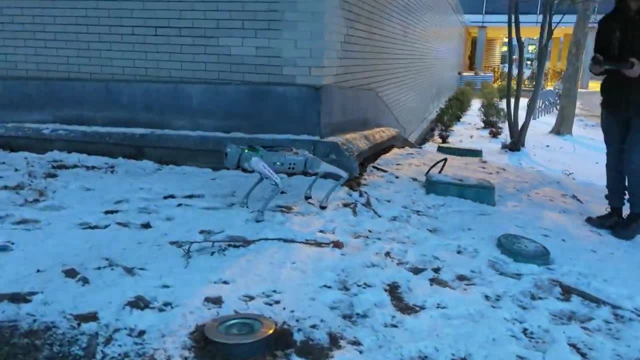 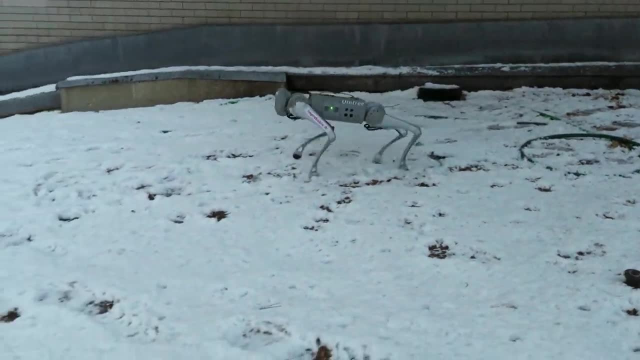 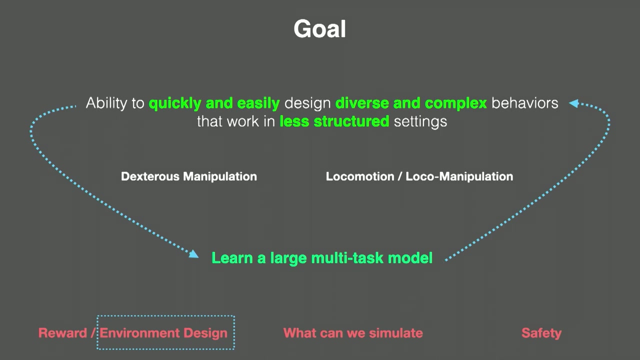 is giving a zero velocity because it is trying to minimize energy. And if you see, we increase the velocity slightly, it moves its legs very little because, again, it's trying to conserve energy. but if you increase velocity it will pick up and, you know, start moving again. So that's something which we are very 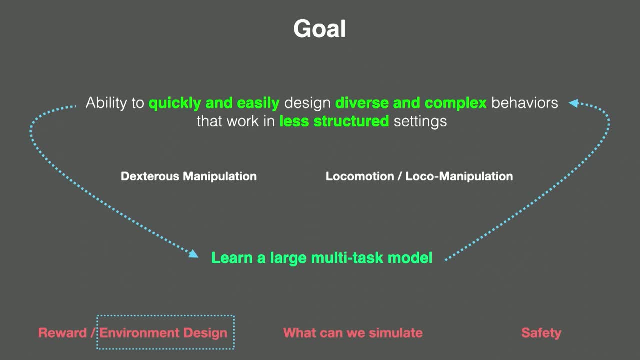 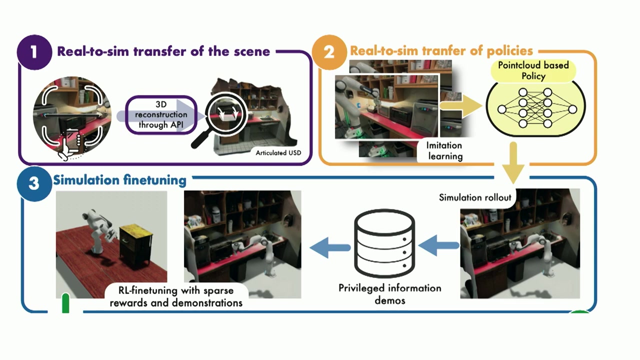 excited about, and I'll just end with the last part, I mean the environment design part, And just someone has to set up the simulation environment and, you know, get assets over there. So in a recent work, you know what we're exploring is, you know, could we scan the real world? you know, with advances which have happened, 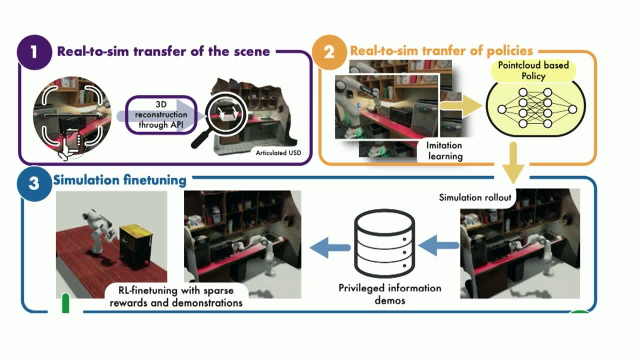 in NERF and other techniques and then add articulations in them, put them into a simulator and then do learning and simulation and again roll them out in reality. So imagine that you have your kitchen and you want to robot to work very well in your kitchen. can you scan your kitchen, put it into a simulator and 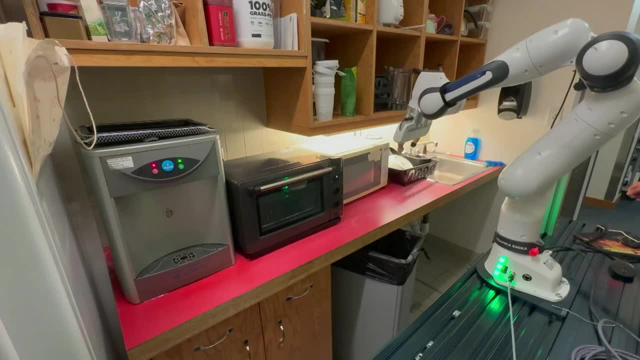 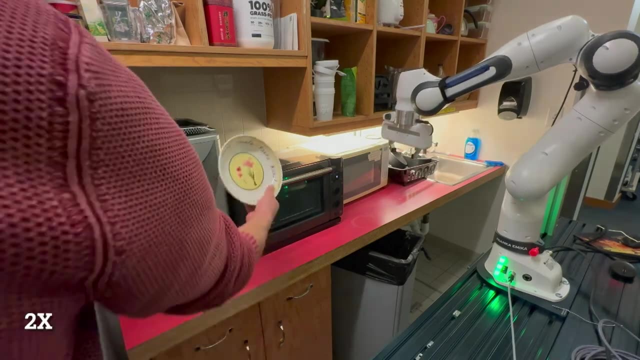 learn policies and put it back in reality. So you know, here's an example of, you know this process, you know which we did in a kitchen in CSAIL, and then you know the goal is to open the microwave and you know Marcel is doing these other 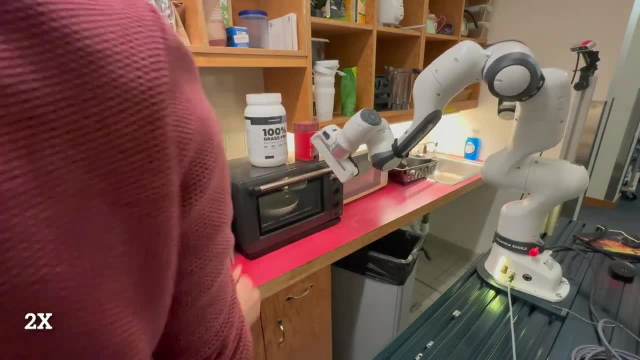 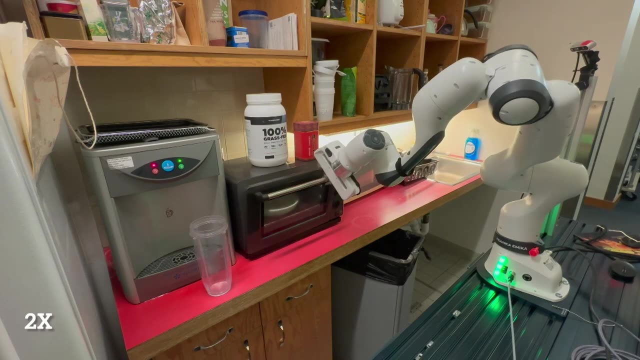 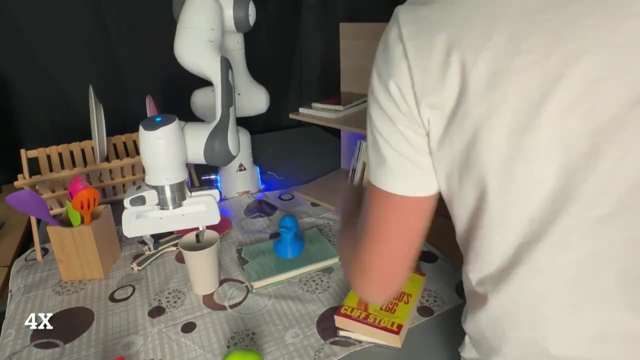 things, while the robot is moving, just to show the robustness which the system has in, you know, performing the task, while other things are happening in background. Even another example over here is that it needs to keep the mug on the shelf, and then we would, you know, move the shelf. you'll see the mug, you know, hit the. 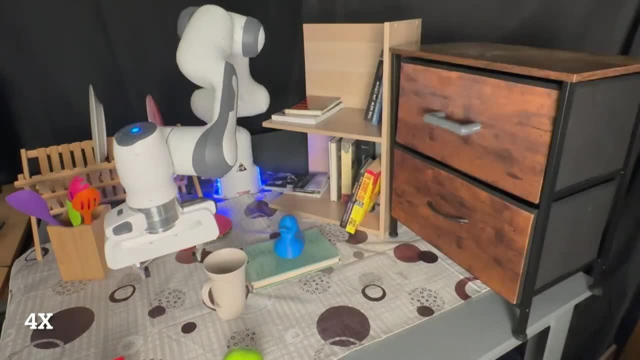 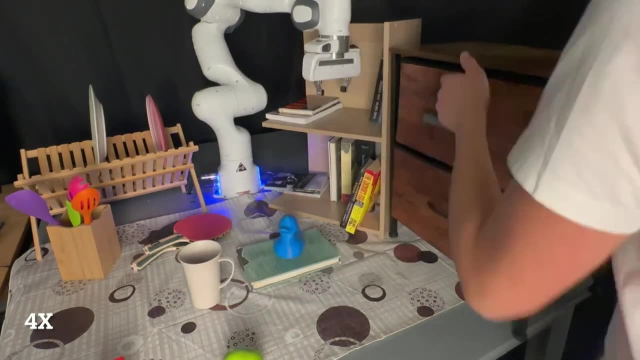 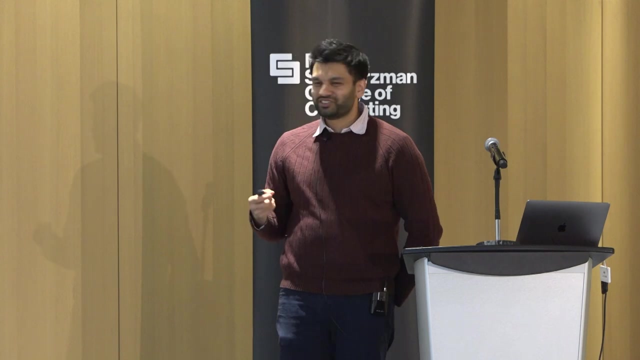 shelf and it is moving. you move the mug back again and the robot will still go and grab it and keep it. So with this, you know, I'll you know, end the talk. You know, if you have, you know, more questions about other aspects. you know about safety, about 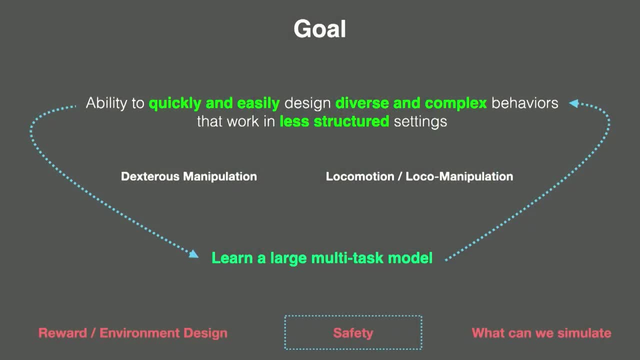 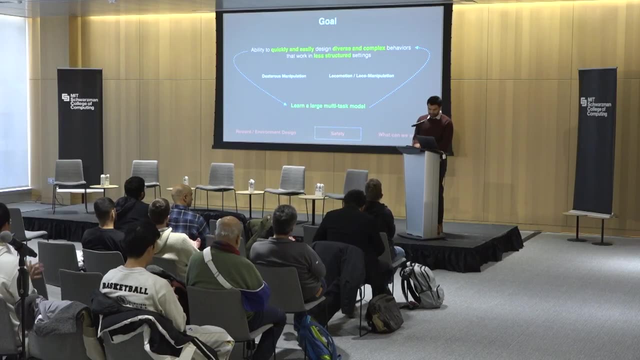 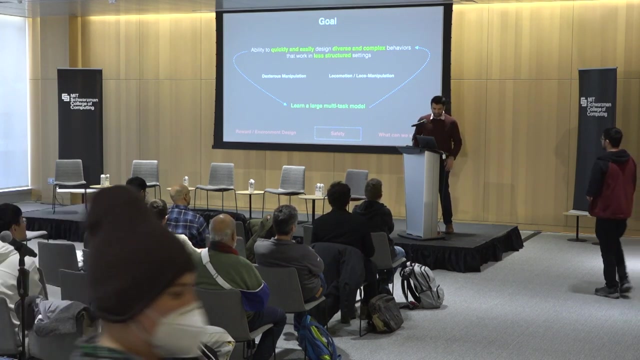 what we can simulate. you know we have some- you know- exciting ongoing work and I'll be happy to chat with you. So thank you so much for your attention. We're going to have to cut it off at 1.30, but if just a couple of questions before then. 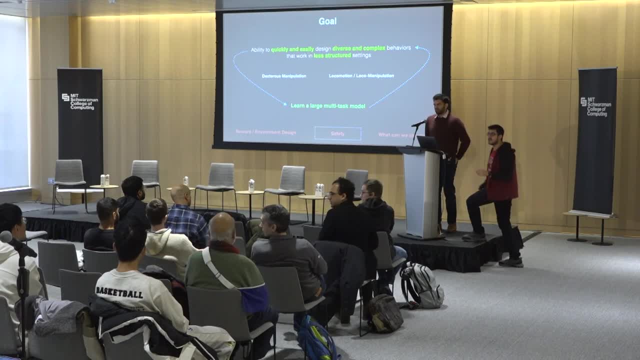 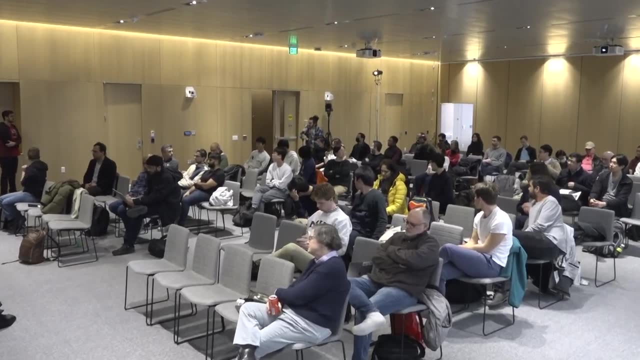 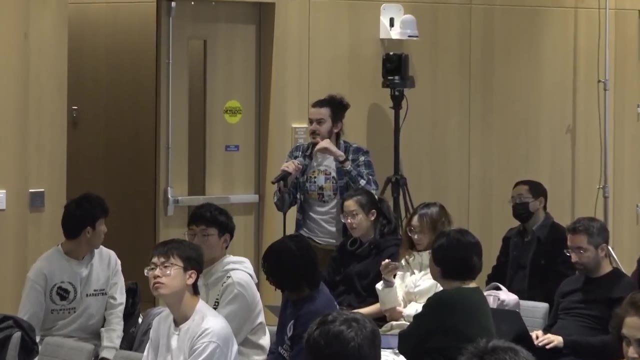 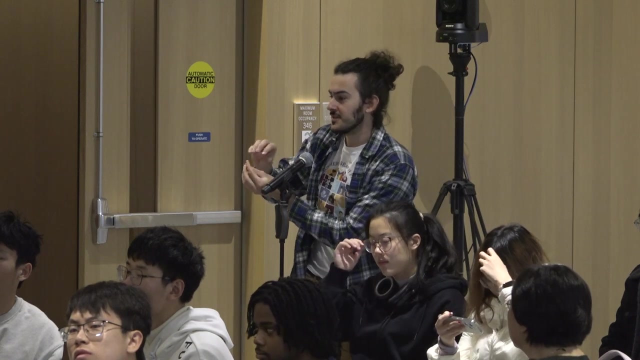 if there's anyone. Hi, thank you for the talk. I was wondering how does this approach generalize to other tasks, or, you know, learning one policy for a certain task and then being able to take sub-skills that it learned in that task to learning another policy more easily? 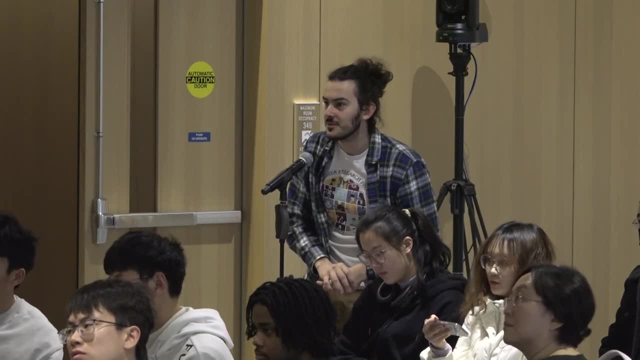 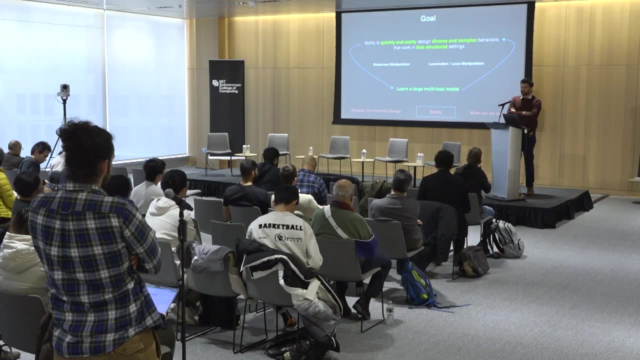 Efficiently. how does that work and what would you need to make that happen? Yeah, so that's something that we have not done yet, right? But, for example, what you would do is you would condition the policy on some identification of the task, right, And that would be the first. 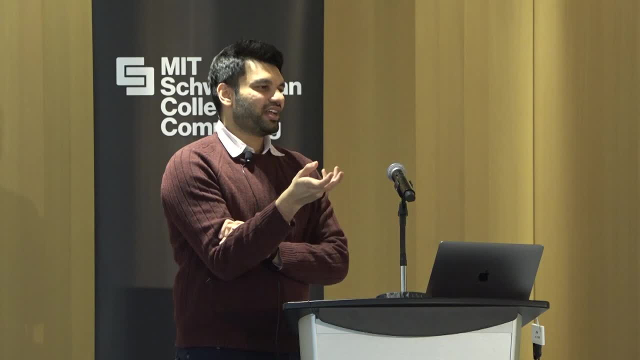 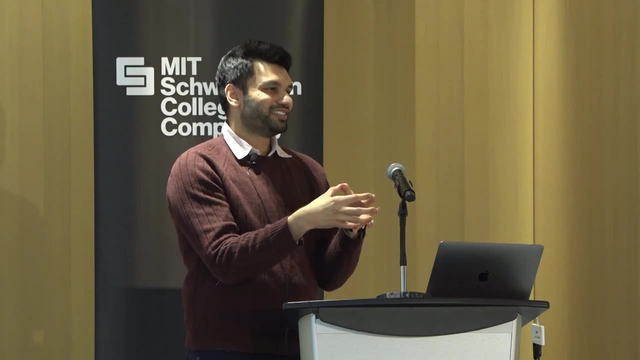 step that you would do And then, if you do that, you know and then you train on multiple tasks, individual policies first, and you can distill them all down into a single model Right. So in the same way as you would expect. 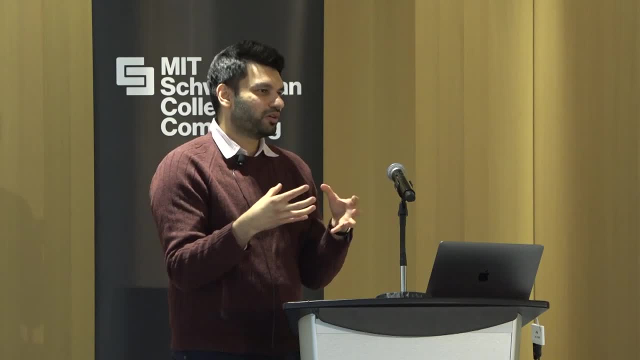 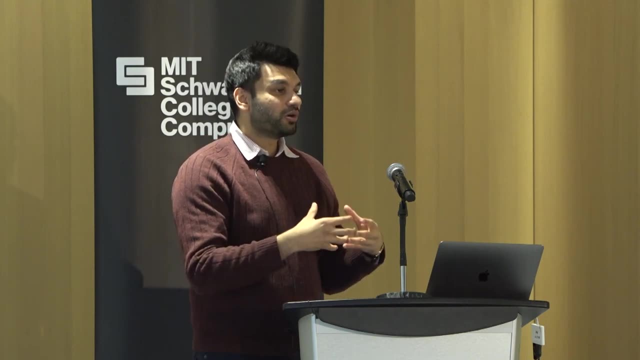 Yeah, Generalization to happen from machine learning. you would, you know, expect the same kind of generalization to happen that now, if you encounter a similar task, you know, then you know the amount of data you might need is going to be lower. And there's a whole different question of how. 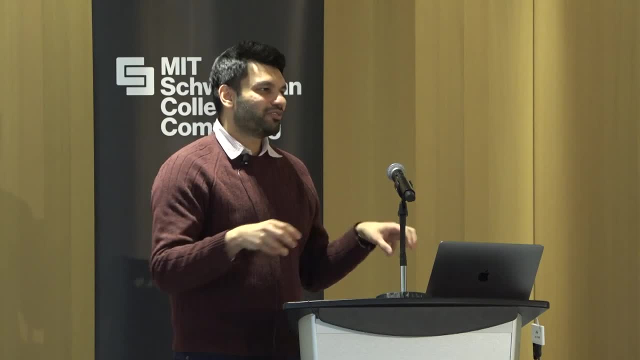 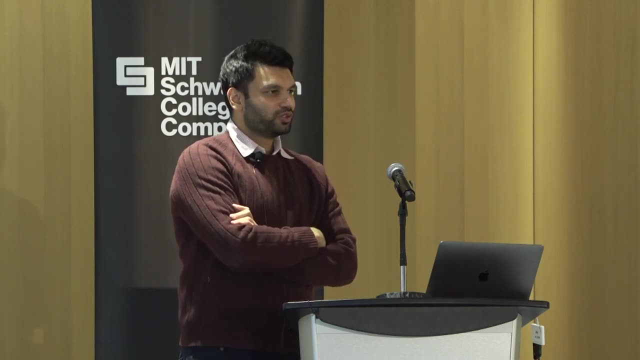 do we plan, you know, using the skills that we already have right. And you know, I think that's a slightly different conversation, because now you need to know when can I execute a particular skill right And when can I not execute a particular skill right. So I think there are formal ways of. 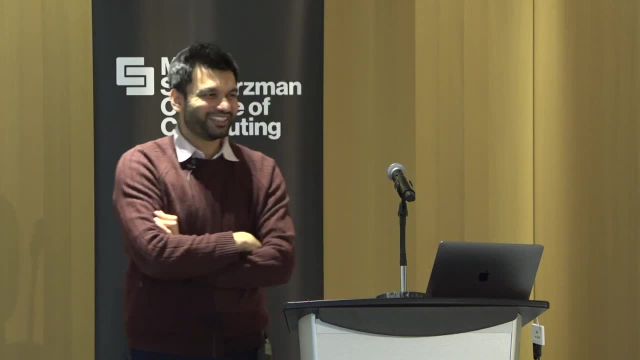 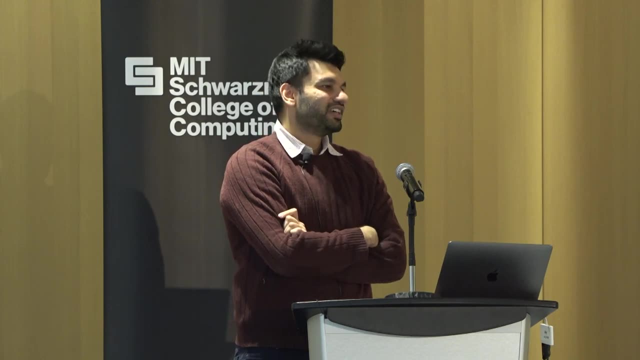 doing it. you know in which Leslie is an expert, And I think there are more machine learning ways of doing it where, for example, in simulation, you can try to learn. you know the distribution of where the skill can start and where the skill will end, right? So I